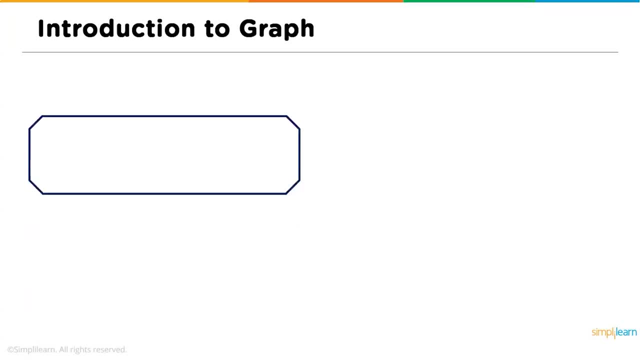 is a brief introduction to graphs. So what exactly is a graph? So a graph is a data structure like any other data structure- example linked list, arrays, etc. So graph is a little different from the other types of data structures, such as linked list and arrays. They are linear. 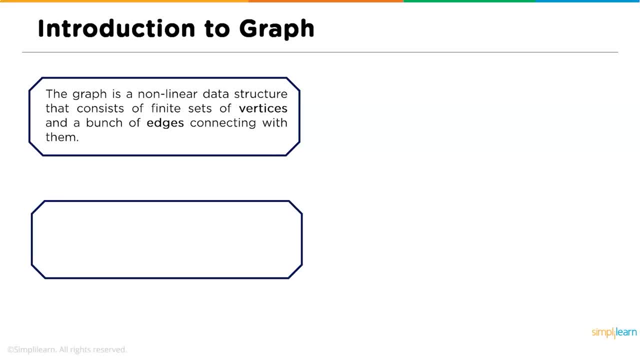 data structures, Whereas graph is a nonlinear data structure that consists of finite sets of vertices and a bunch of edges connecting with them. So what are these vertices and edges? So let us understand that a graph is usually represented by a set of vertices and edges, So a vertex is the node present in a graph. Imagine that. 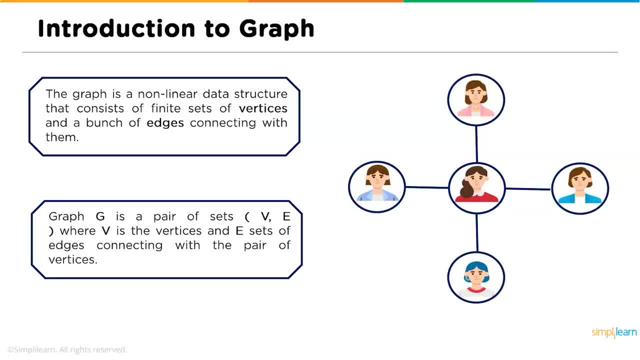 you are a group of five friends, So each one of you is considered as a vertex and the network connecting you guys is known as an edge. So the overall graph of you people can be considered as an edge And it is represented by vertices and edges set where vertices is you and the. 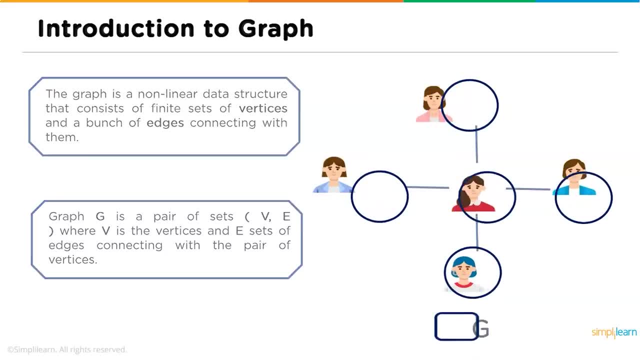 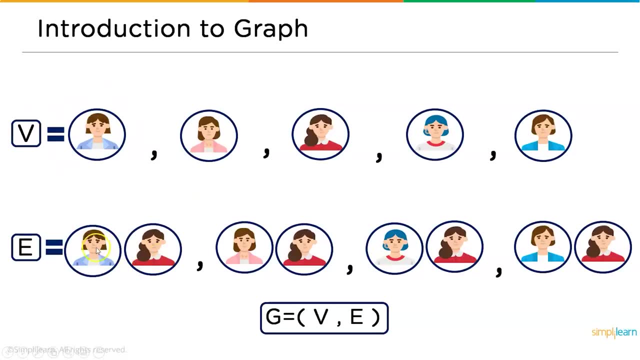 network connecting you guys is called as an edge. So here you can see it clearly: Each one of the friends is called as a vertex and the network connecting them is called as an edge, And the entire graph is represented using a set of vertices and edges. Now moving. 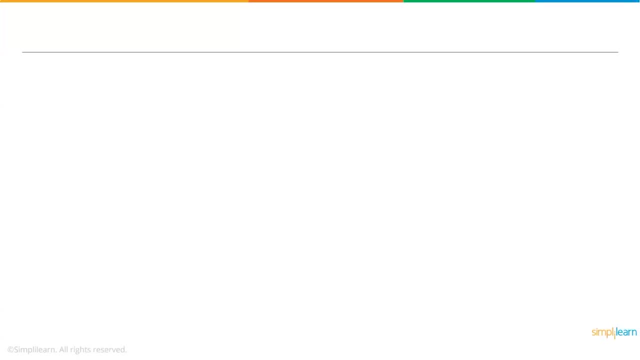 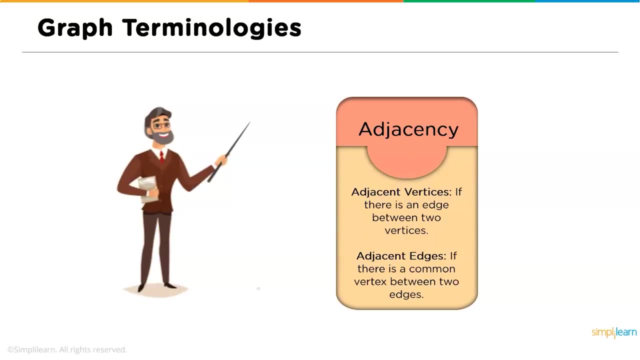 ahead. we will understand the graph terminologies Now. at first we have the adjacency vertices and adjacency edges. So what are adjacent vertices? if there is an edge between two vertices, That is, one vertex or one node is connected to another node directly using just one single edge, Then those vertices are called as adjacent. 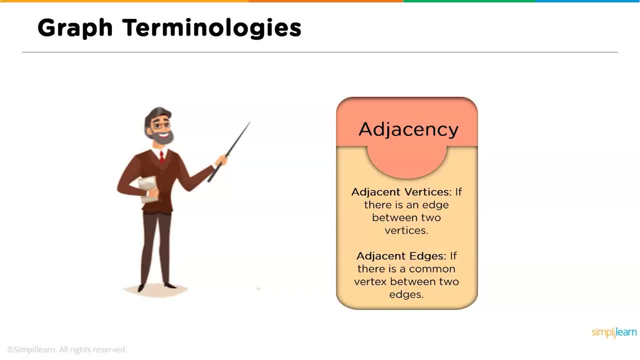 vertices. Now, what are adjacent edges? If there is one common, whether its between two edges, edges are called as adjacent edges. Let's imagine this way. Let us imagine that we have three vertices and these three vertices are connected using two edges. So here we have one vertex, which 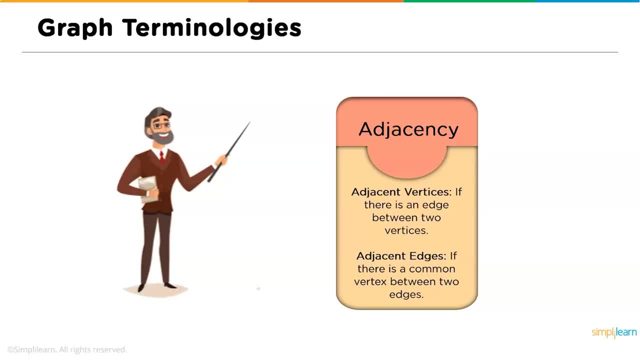 is common between these two edges, So such type of edges are called as adjacent edges. Next we have the degree. In an undirected graph, number of vertices adjacent to the vertex is called as a degree. Next is the path. The path is considered as a sequence of distinct vertices. 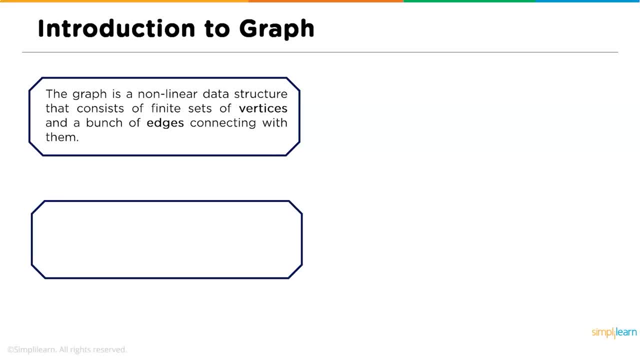 data structures, Whereas graph is a nonlinear data structure that consists of finite sets of vertices and a bunch of edges connecting with them. So what are these vertices and edges? So let us understand that a graph is usually represented by a set of vertices and edges, So a vertex is the node present in a graph. Imagine that. 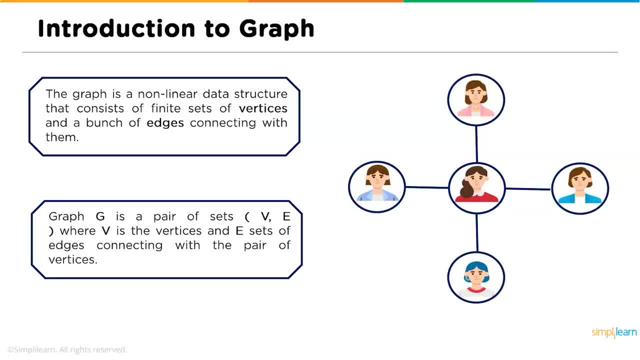 you are a group of five friends, So each one of you is considered as a vertex and the network connecting you guys is known as an edge. So the overall graph of you people can be considered as an edge And it is represented by vertices and edges set where vertices is you and the. 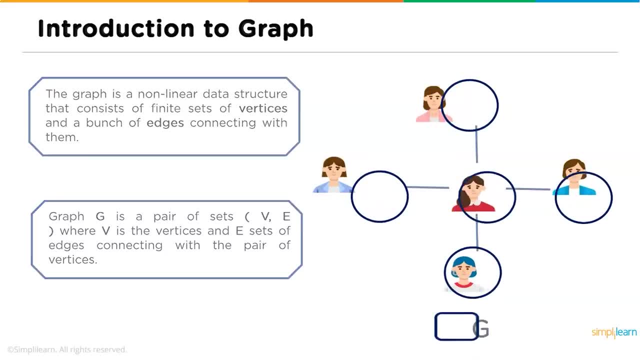 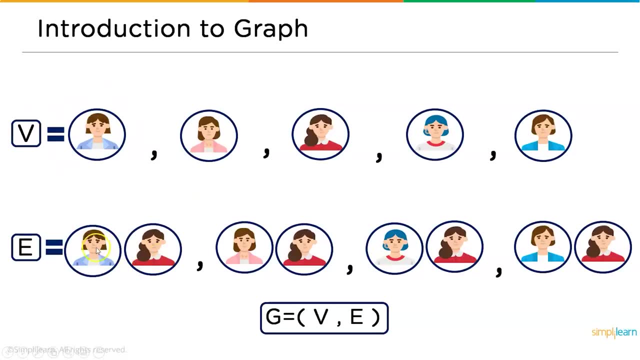 network connecting you guys is called as an edge. So here you can see it clearly: Each one of the friends is called as a vertex and the network connecting them is called as an edge, And the entire graph is represented using a set of vertices and edges. Now moving. 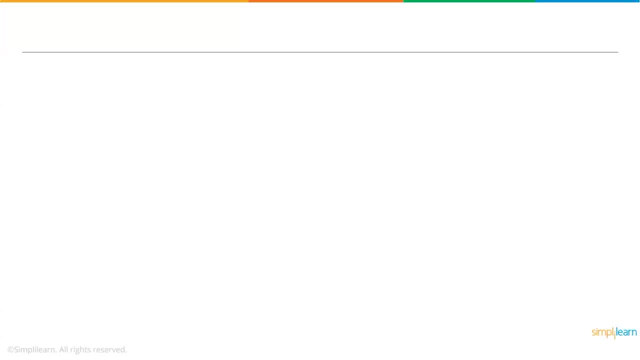 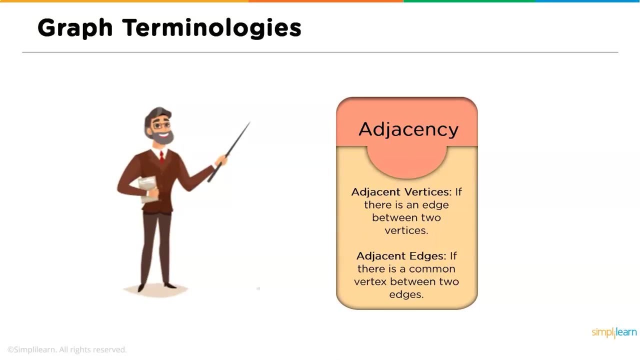 ahead. we will understand the graph terminologies Now. at first we have the adjacency vertices and adjacency edges. So what are adjacent vertices? If there is an edge between two vertices, that is, one vertex, or one node is connected to another node directly using just one single edge, then those vertices are called as adjacent. 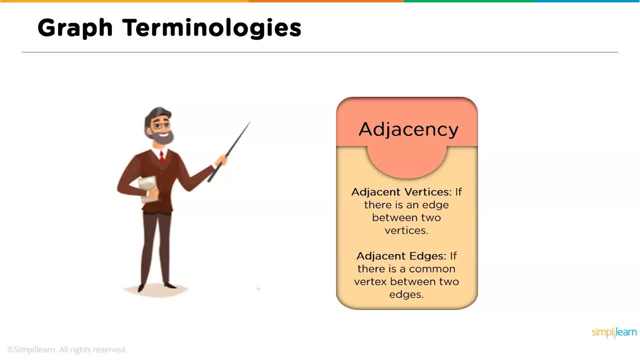 vertices. Now, what are adjacent edges? If there is one common vertex between two edges, then those two edges are called as adjacent edges. Let us imagine this way. Let us imagine that we have three vertices and these three vertices are connected using two edges. So 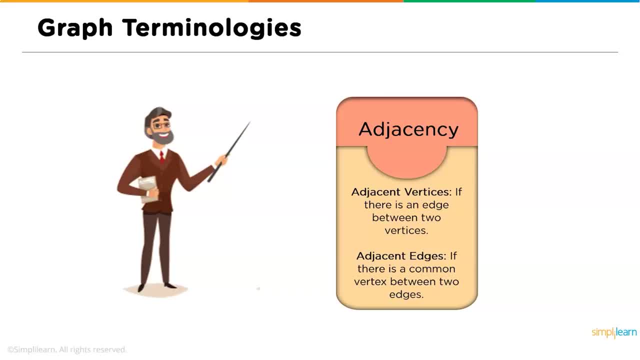 here we have one vertex which is common between these two edges, So such type of edges are called as adjacent edges. Next we have the degree. In an undirected graph, number of vertices adjacent to the vertex is called as a degree. Next is the 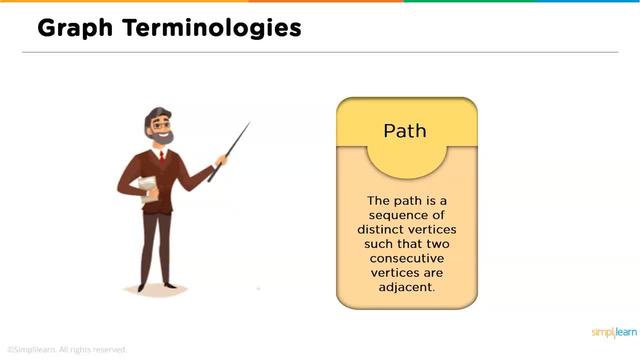 path. The path is considered as a sequence of distinct vertices, such that two consecutive vertices are adjacent to each other. Up next we have the cycle, A path that has only one. repeated vertices are called as first and last vertices. Followed by that, we have the walk. 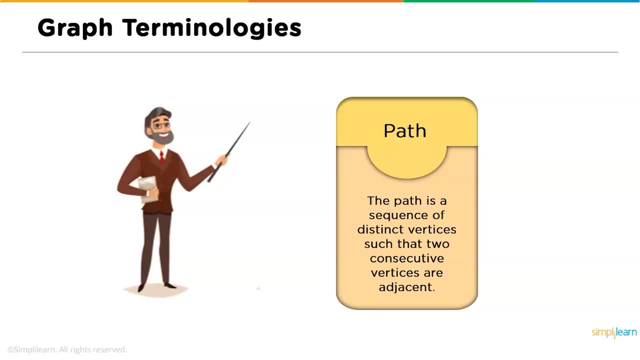 such that two consecutive vertices are adjacent to each other. Up next we have the cycle, A path that has only one. repeated vertices are called as first and last vertices. Followed by that we have the walk. The term walk is self-explanatory. A walk is the sequence of 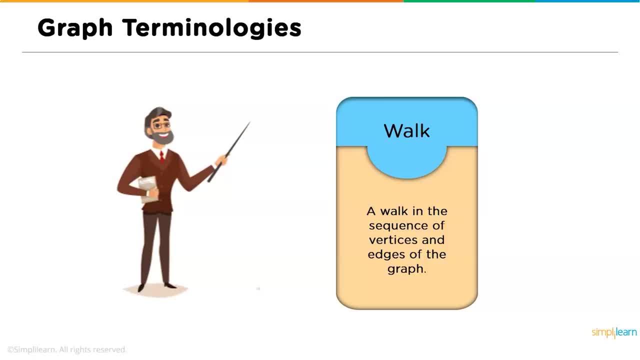 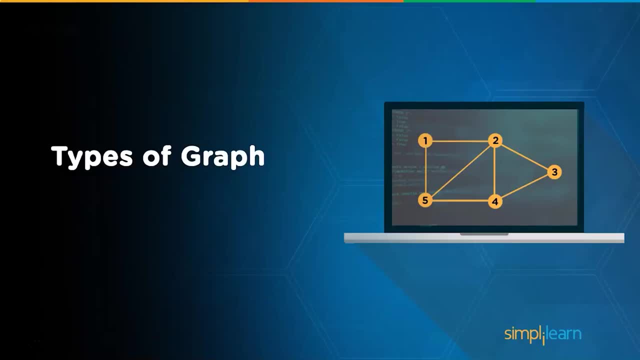 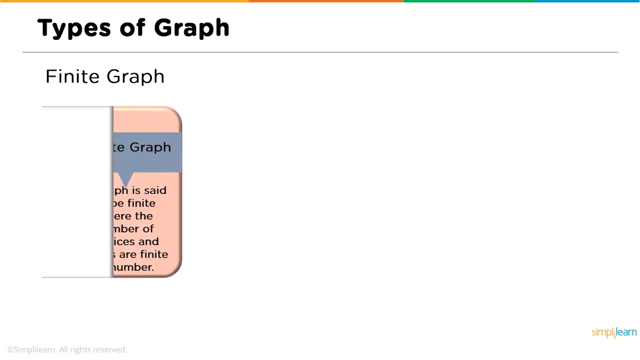 vertices and edges In the graph, which is used to traverse through one vertex to another vertex. Now we have entered the next segment of this particular tutorial, where we will be discussing the different types of graphs available. So at first we have the finite graph. So what exactly? 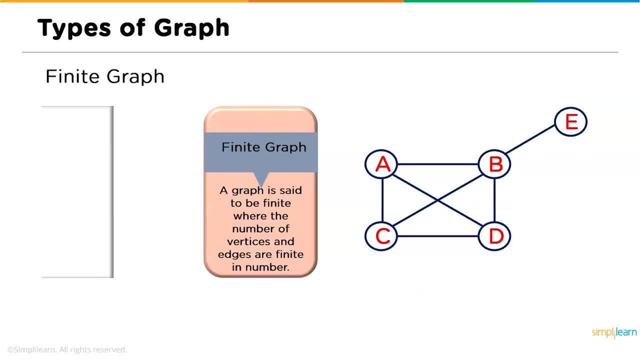 is a finite graph. A graph is said to be finite when the number of vertices and the number of edges are in a finite number or in a countable number. Now, the next type of graph is the infinite graph. So what exactly is the infinite graph? 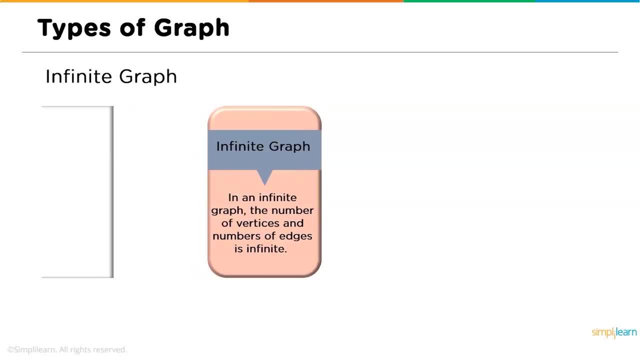 So the infinite graph is a typical opposite of the finite graph. So this particular graph will not have countable number of edges and countable number of vertices. The image here is an example for a typical infinite graph. Now, followed by the infinite graph, we have the trivial graph. 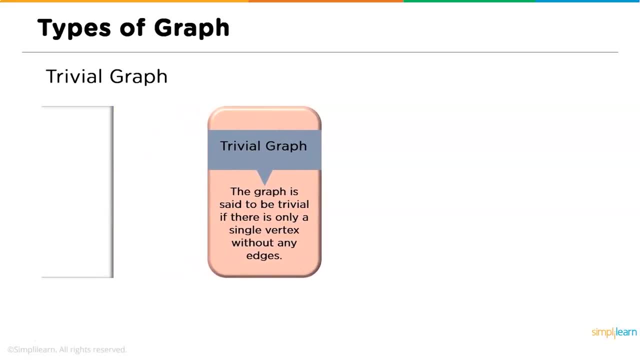 So what is a trivial graph? A graph is said to be trivial if there is only one single vertex, without any edges. So this particular type of graph will only have vertex. that is, only one single vertex, not more than one, and there will be no edge. If you have just one vertex, then there is. 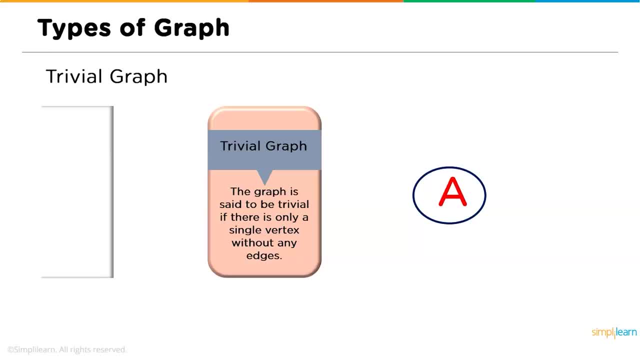 no possibility of having an edge, Unless if you have one single loop type of edge which is connecting to itself. But in a trivial graph we do not even have that. We just have one single vertex. So, followed by trivial graph, we have a simple graph. 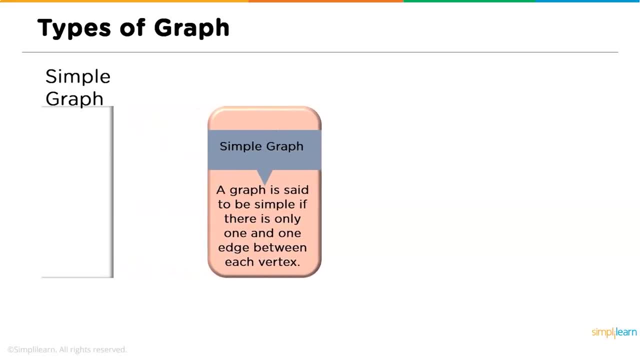 So what exactly is a simple graph? A graph is said to be simple if there is only one and one edge between each vertex. So this particular example can be considered as a simple graph. So here, each and every set of vertices have one single edge between them. 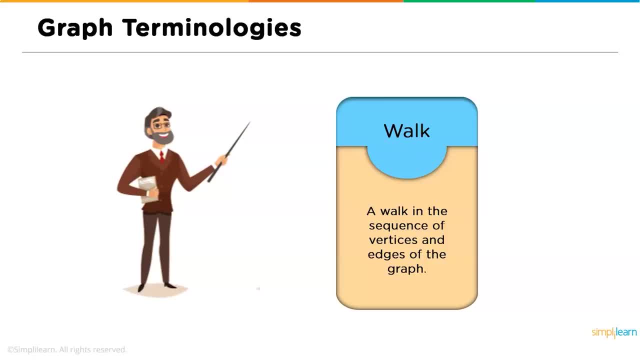 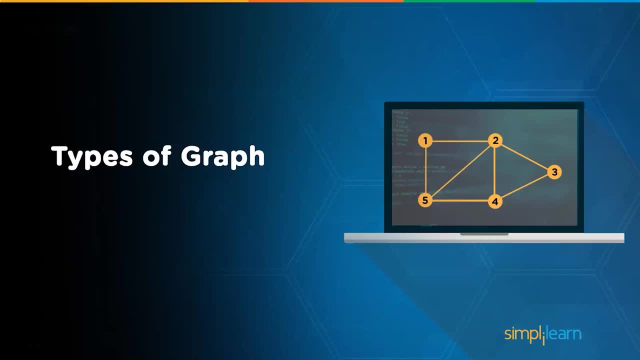 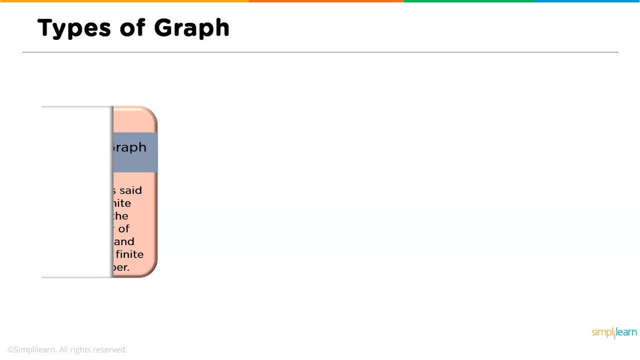 The term walk is self-explanatory. A walk is the sequence of vertices and edges in the graph which is used to traverse through one vertex to another vertex. Now we have entered the next segment of this particular tutorial, where we will be discussing the different types of graphs available. So at first we have the finite graph. 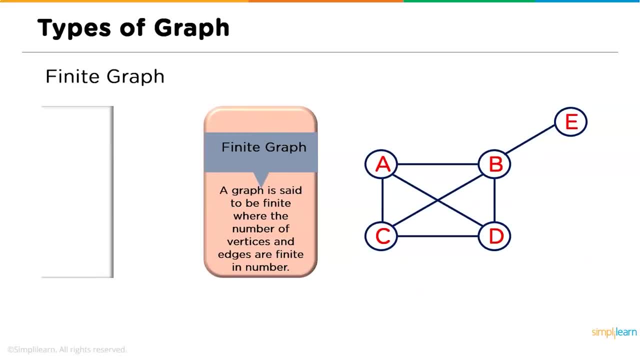 So what exactly is a finite graph? A graph is said to be finite when the number of vertices and the number of edges are in a finite number or in a countable number. Now let's look at the finite graph. A graph is said to be finite when the number of vertices and the number of edges are in a countable number. 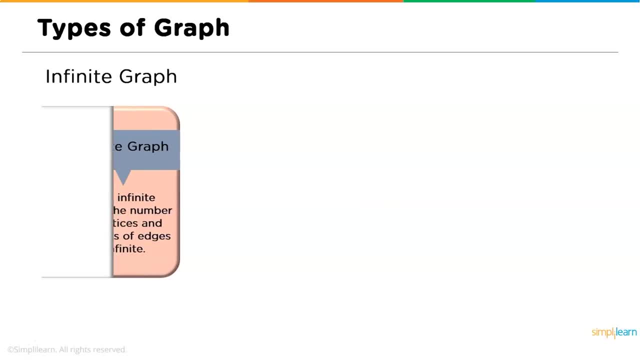 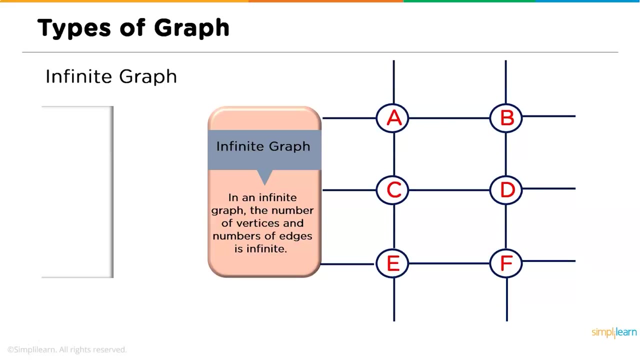 Now the next type of graph is the infinite graph. So what exactly is the infinite graph? So the infinite graph is a typical opposite of the finite graph. So this particular graph will not have countable number of edges and countable number of vertices. The image here is an example for a typical 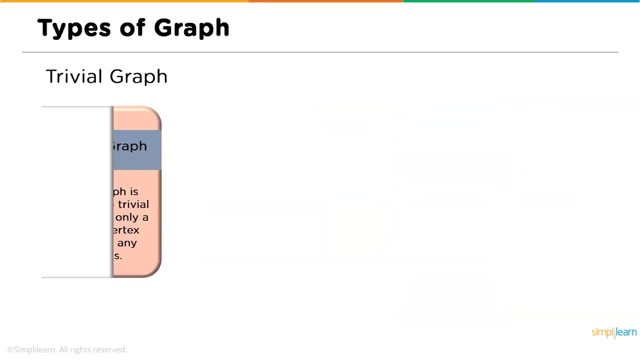 infinite graph. Now, followed by the infinite graph, we have the trivial graph. So what is a trivial graph? A graph is said to be trivial if there is only one single vertex, without any edges. So this particular type of graph will only have vertex, that is, only one single vertex, not more than one, and there will be no edge. 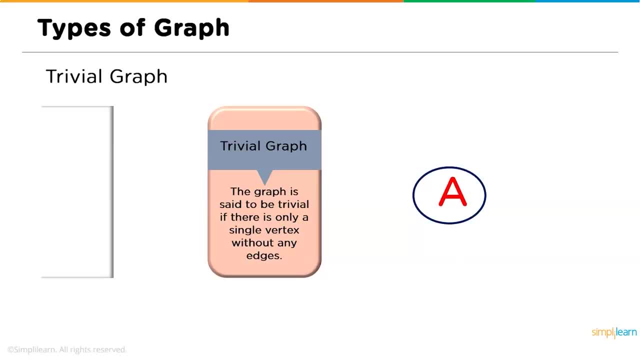 If you have just one vertex, then there is no possibility of having an edge, unless if you have one single loop type of edge which is connecting to itself. But in a trivial graph we don't even have that. We just have one single vertex, So followed by trivial 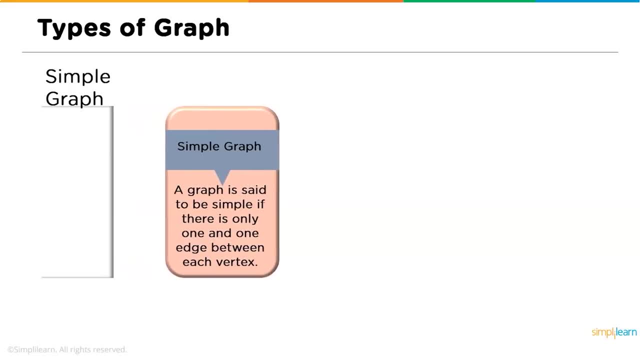 graph. we have a simple graph. So what exactly is a simple graph? A graph is said to be simple if there is only one and one edge between each vertex. So this particular example can be considered as a simple graph. So here, each and every set of vertices have 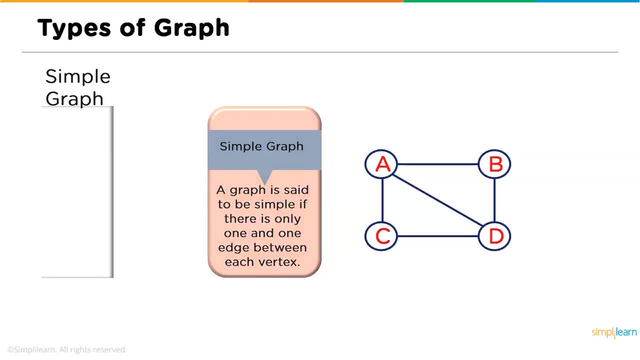 one single edge between them. Now, followed by the simple graph, we have the multi graph. So if there are multiple edges between the pair of vertices, then this particular type of graph is known as a multi graph. So here you can see that we have two vertices, a and b, and we have two edges connecting. 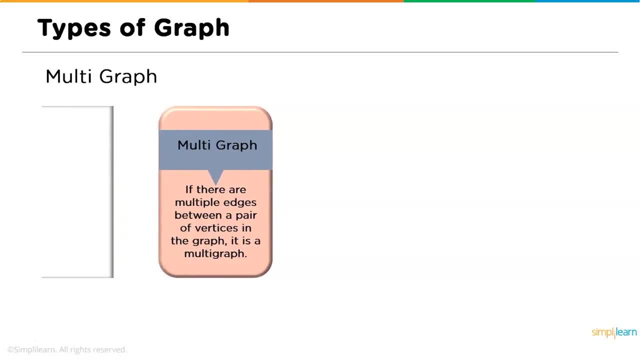 Now, followed by the simple graph, we have the multi graph. So if there are multiple edges between the pair of vertices, then this particular type of graph is known as a multi graph. So here you can see that we have two vertices, A and B, and we have two edges connecting. 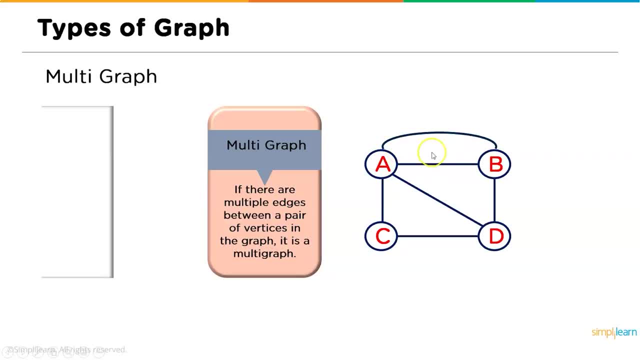 them Not one but two. But in a simple graph we were supposed to have just one edge connecting the vertices. So this is the difference between simple graph and a multi graph. So, followed by multi graph, we have a null graph. 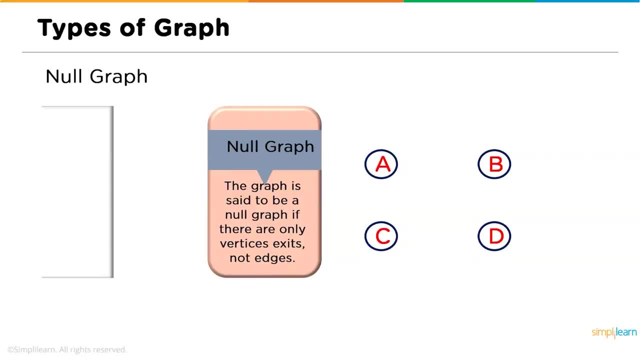 So what is a null graph? A graph is said to be null if there are only vertices and no edges between them. So remember the trivial graph: right, We just had one single vertex but no edges. But here we do have multiple vertices, but no edges connecting them. 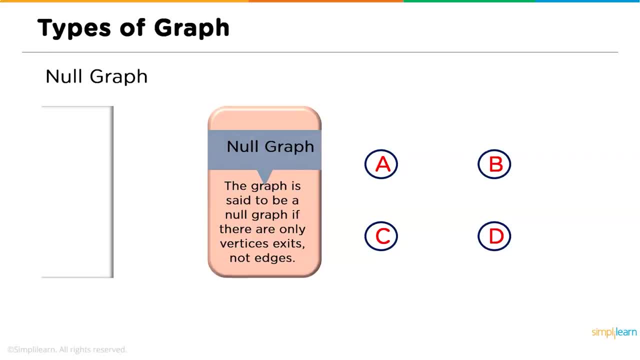 So this type of a graph is considered as a null graph. So, followed by a null graph, we have the complete graph. So what is a complete graph? A graph is called as a complete graph, where each vertex must be connected with the other. 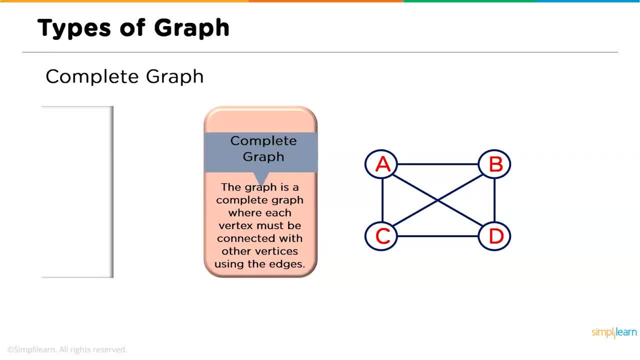 vertices using the edges. So the meaning of this particular graph is that each vertex must be connected with the other vertices using the edges. So the meaning of this particular type of graph is: all the edges are connected to all the other edges using at least one single edge. 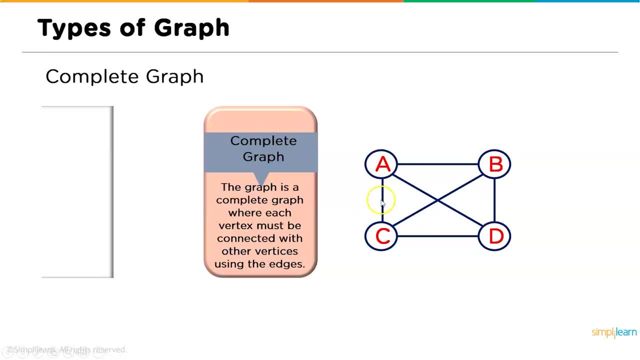 So here you can see, A is connected to B, D and C, all together with at least one edge, And similarly, all other vertices are connected to each other with at least one single edge. Now, followed by the complete graph, we have the pseudograph. 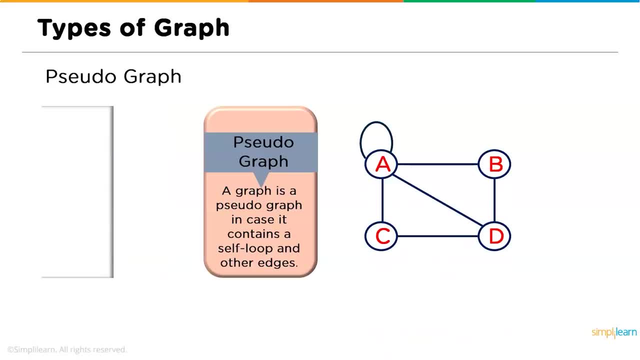 So what is a pseudograph? A pseudograph is a graph where at least one vertex will have seven edges. So what is a pseudograph? A pseudograph is a graph where at least one edge or any other type of edge will have. 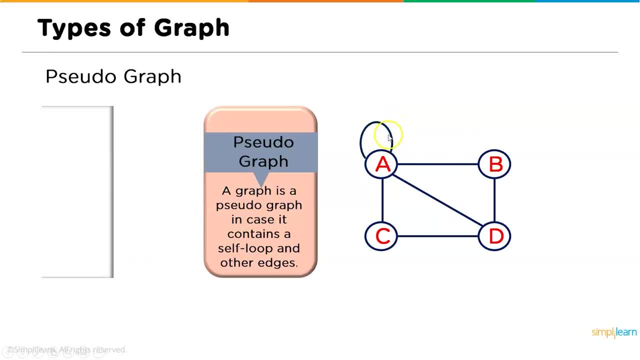 six of six edges, and each of these eight edges will have 12 edges. These individual edges are linked to a pewner. They look like aSPEAKING on a новые oder. Whenever you try to send an image, you end up sending a video with a few hours of old. 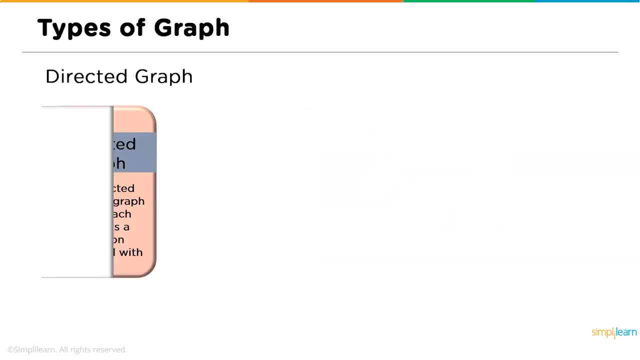 images like that. So because this is a pseudograph. a pseudograph is a graph where you end up sending a новr ghost. The businesses do not look like this any more. Any flashcards should not be salute text graph where each edge has a direction associated with it. So so far, we have just discussed the 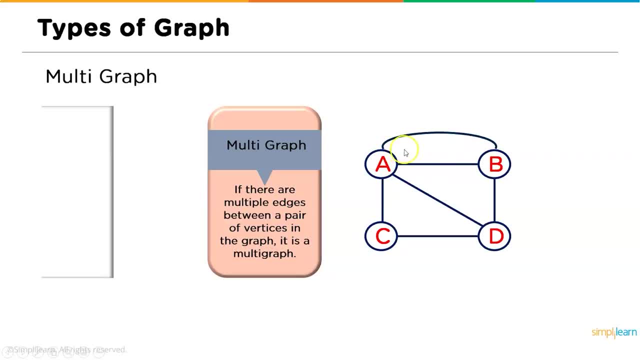 them not one but two. But in a simple graph we were supposed to have just one edge connecting the vertices. So this is the difference between simple graph and a multi graph. So, followed by multi graph, we have a null graph. So what is a null graph? A graph is: 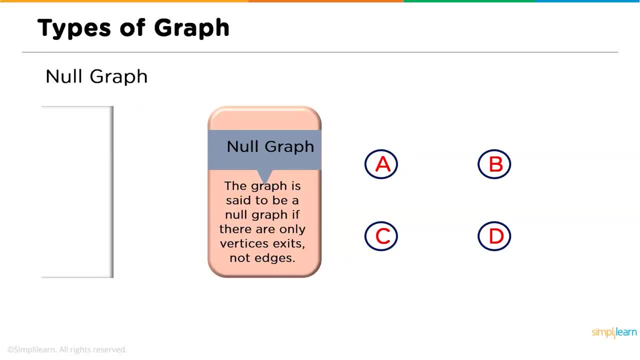 said to be null if there are only vertices and no edges between them. So remember the graph: right, We just had one single vertex but no edges. But here we do have multiple vertices but no edges connecting them. So this type of a graph is considered as a 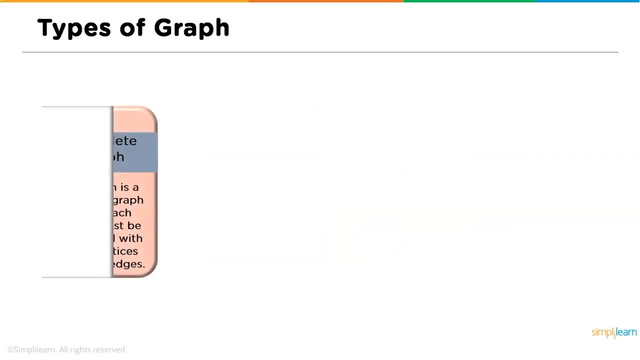 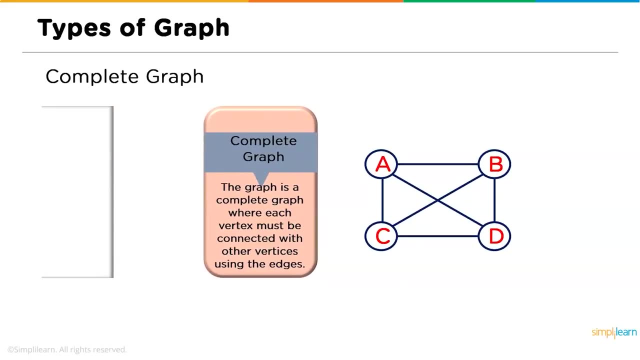 null graph, So, followed by null graph, we have the complete graph. So what is a complete graph? A graph is called as a complete graph, where each vertex must be connected with the other vertices using the edges. So the meaning of this particular type of graph. 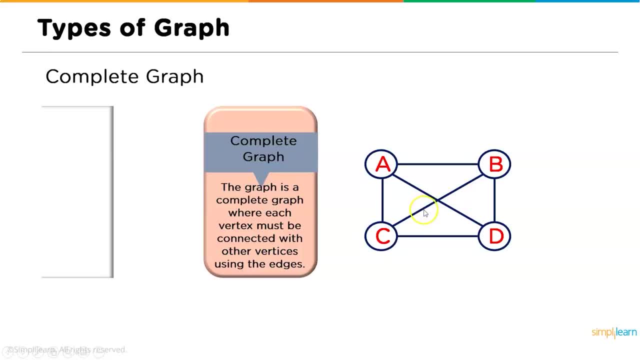 all the edges are connected to all the other edges using at least one single edge. So here you can see: a is connected to b, d and c, all together with at least one edge, and similarly, all other vertices are connected to each other with at least one single edge. 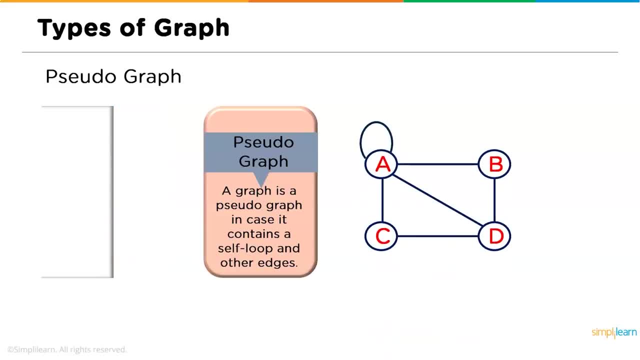 Now, followed by the complete graph, we have the pseudo graph. So what is a pseudo graph? A pseudo graph is a graph where at least one vertex will have self looping type of edge. Self loop or self edge we have discussed in the trivial graph type. So this particular 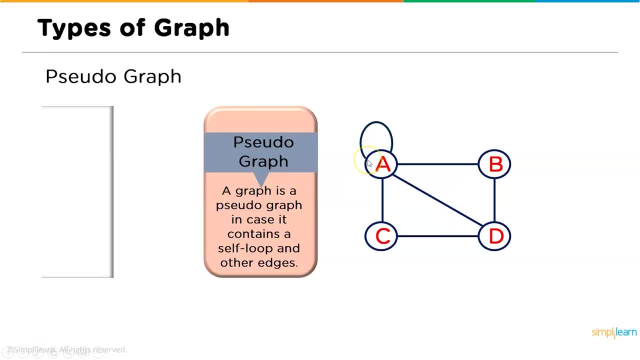 type of an edge where it connects to itself is called as a loop or kind of self connecting edge. So any graph that has this kind of a edge is called as a pseudo graph. So, followed by the pseudo graph, we have the directed graph. So what is a directed graph? 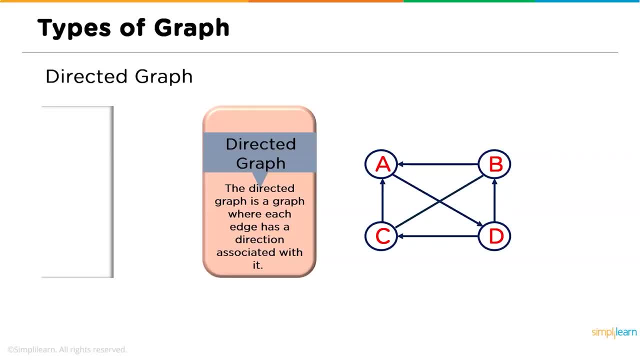 Any graph is called as a directed graph, where each edge has a direction associated with it. So so far we have just discussed the edges which are connecting to one or the other vertex, but there was no direction. But here you can see that this particular edge has a direction that is from b to a, not from a to b, it is from b to a. 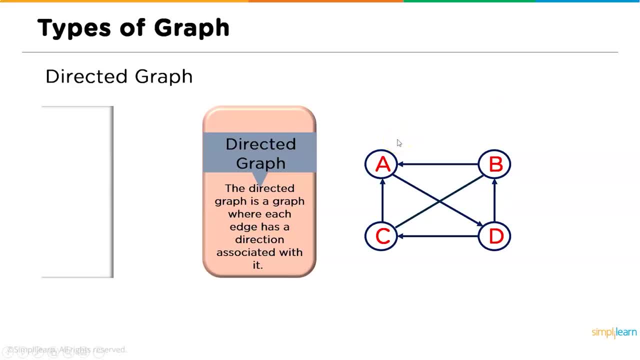 edges which are connecting to one or the other vertex, but there was no direction. but here you can see that this particular edge has a direction that is from B to A, not from A to B, it is from B to A. This type of edges, which are directing the traversal of the graph, are known as the directed. 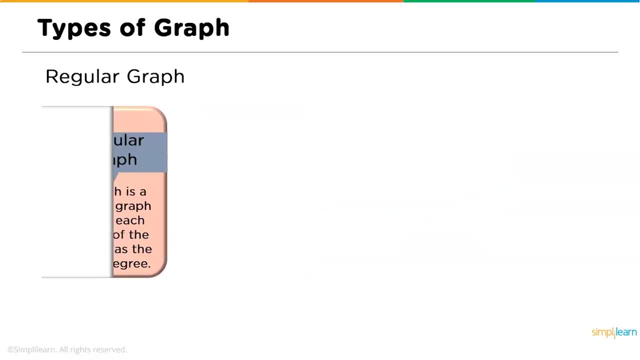 graphs. Now, followed by the directed graphs, we have the regular graph. So a graph is a regular graph where each vertex of the graph has the same degree. Now, here you can see, all the vertices have the same amount of degree. that is the connection between all the other vertices. So the degree of 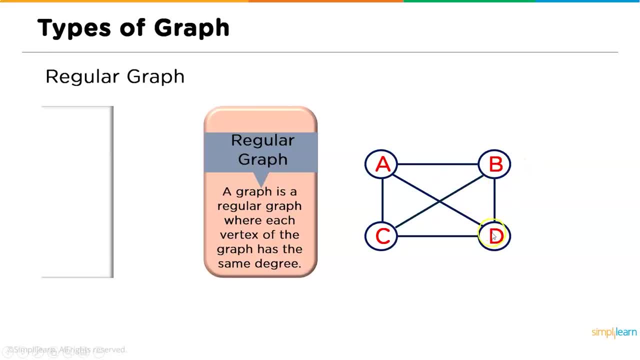 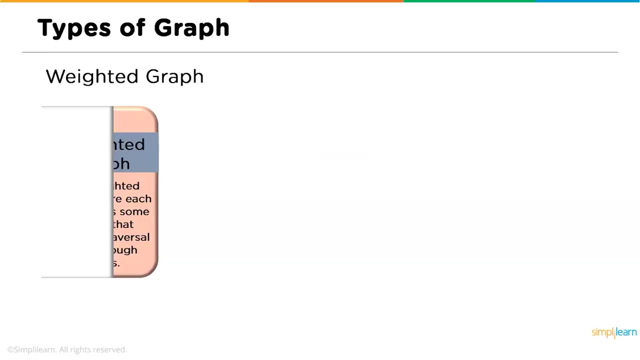 A is 3.. So the degree of B is also 3, and the degree of D is C, and similarly the degree of C is also 3.. So what I mean to say is all of these vertices have the same degree, that is, 3.. Now we have the weighted graph, So 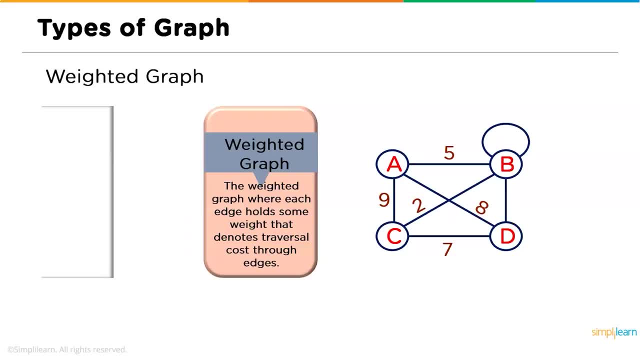 what is a weighted graph? A weighted graph is where each edge holds some weight that denotes the traversal caused through those edges. Now, here you can see that all the edges have a different weight. The edge from A to B has the weight 5, and the edge from A to C has the weight 9 and the 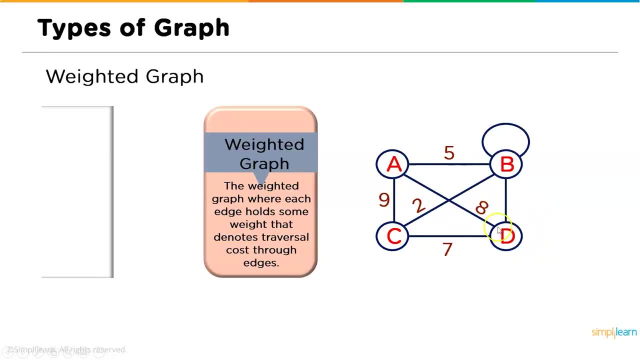 edge from C to B has 2.. So the edge from A to B has the weight 9 and the edge from C to B has the weight 2 and the edge A to D has 8 and finally C to D has 7.. So all these values are the weight or the cost. 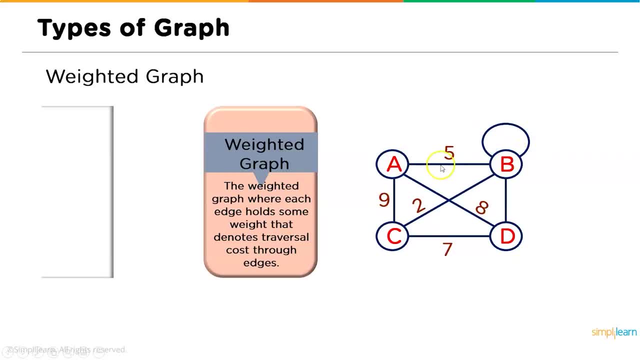 to traverse from A to another vertex flow. So from A to B, we have the cost 5, and A to C, we have the cost 9, and similarly C to D, we have 7 and so on. Now, followed by the weighted graph, we have the. 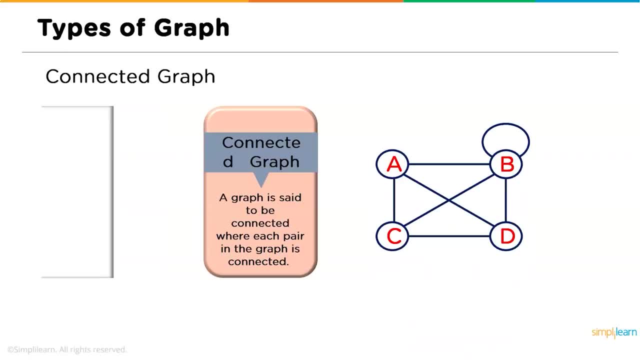 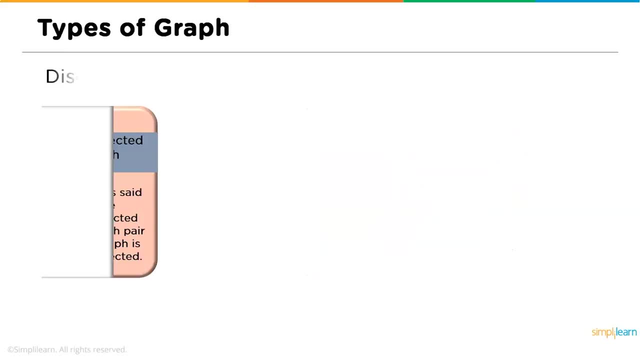 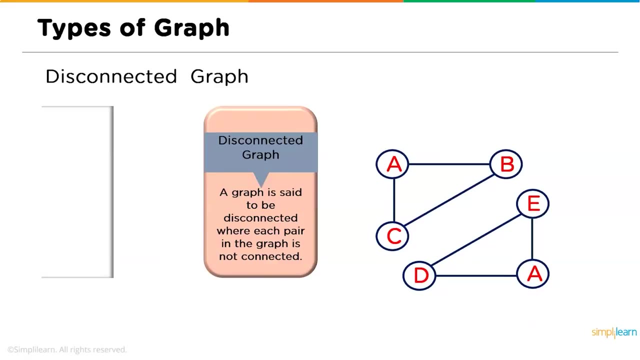 connected graph. So what exactly is a connected graph? A graph is said to be connected where each pair in the graph is connected, Followed by a connected graph. we have the disconnected graph. So it is a typical opposite of the connected graph. A graph is said to be disconnected where each pair in the graph is not. 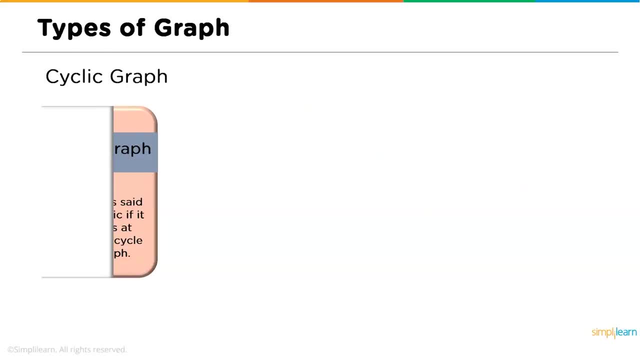 connected to each other. Now, next, we have the cyclic graph. So a graph is said to be cyclic if it contains at least one cycle in a graph, that is one complete traversal connection. So A can be traversed again from traveling A to C. 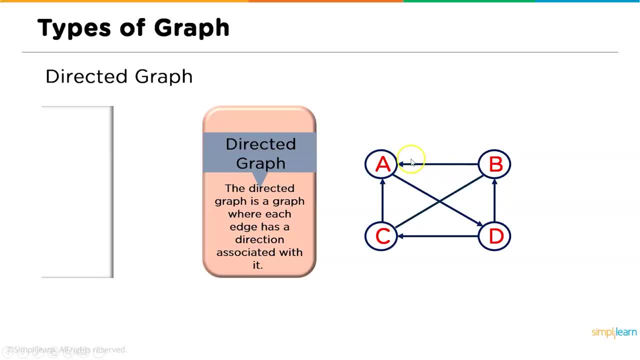 This type of edges, which are directing the traversal of the graph, are known as the directed graphs. Now, followed by the directed graphs, we have the regular graph. So a graph is a regular graph Where each vertex of the graph has the same degree. Now, here you can see all the vertices. 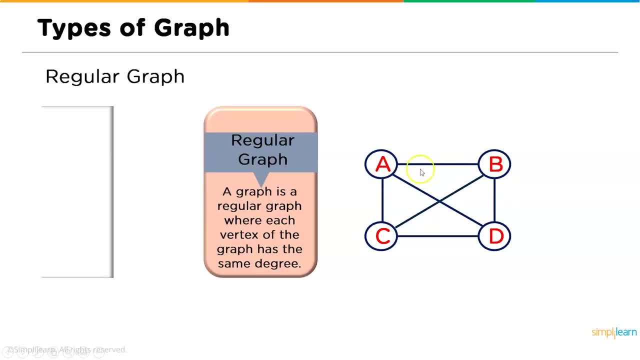 have the same amount of degree. that is the connection between all the other vertices. So the degree of a is 3, so the degree of b is also 3, and the degree of d is c and similarly the degree of c is also 3.. So what I mean to say is all of these vertices have the same. 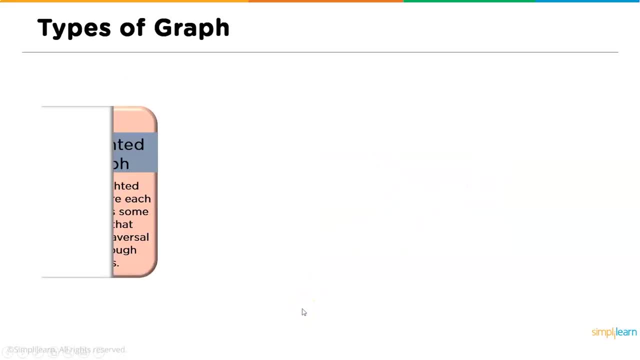 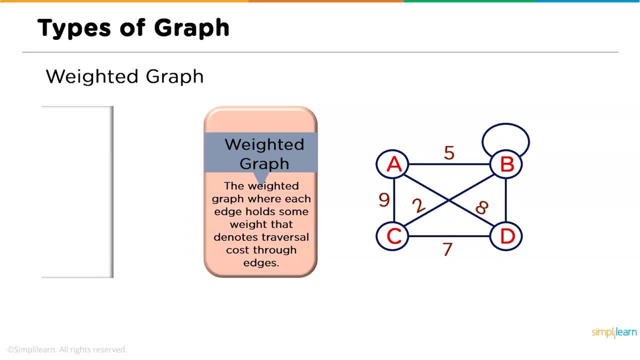 degree, that is 3.. Now we have the weighted graph. So what is a weighted graph? A weighted graph is where each edge holds some weight. that denotes the traversal course through those edges. Now, here you can see that all the edges have a different weight. The edge from a to b has 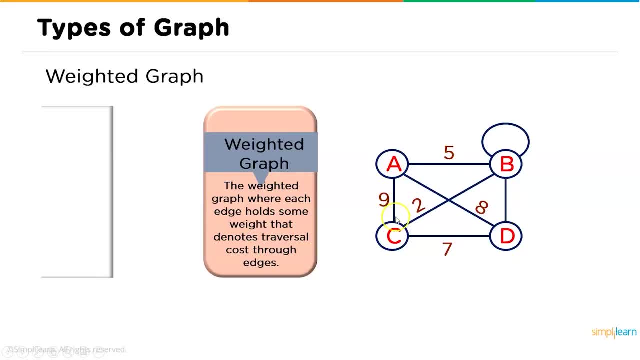 the weight 5 and the edge from a to c has the weight 9, and the edge from c to b has 2 and the edge from a to d has 8 and finally, c to d has 7.. So all these values are the. 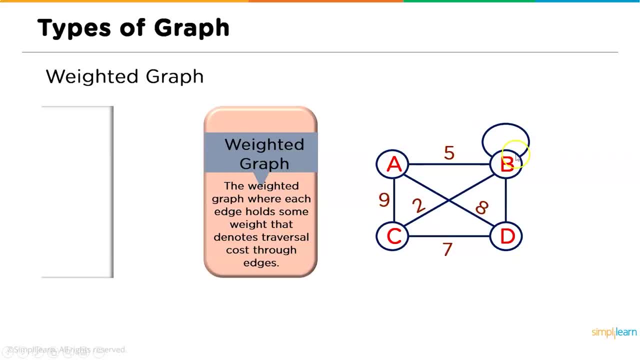 weight or the cost to traverse from A to another vertex flow. So from A to b, we have the cost 5, and from A to c we have the cost 9, and similarly from c to d we have 7, and so on. Now, followed by the weighted graph, we have the connected graph. 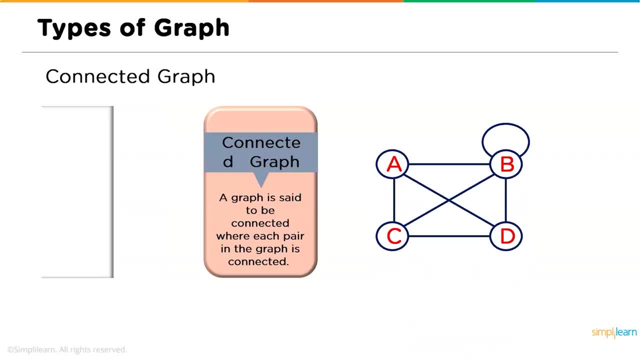 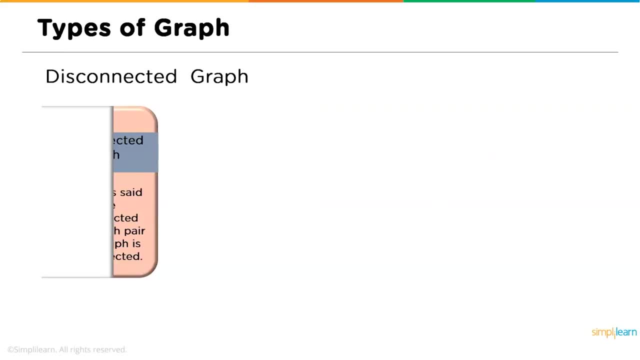 So what exactly is a connected graph? A graph is said to be connected when each pair in the graph is connected, Followed by a connected graph. We have the disconnected graph. So it is a typical opposite of the connected graph. Yeah, graph, a graph is said to be disconnected where each pair in the graph is not connected to each. 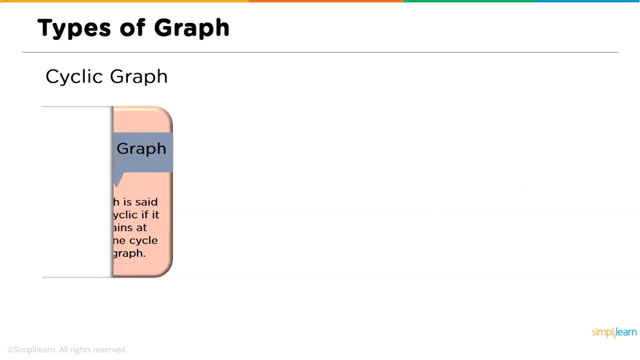 other Now. next we have the cyclic graph. So a graph is said to be cyclic if it contains at least one cycle in a graph, that is one complete traversal connection. So A can be traversed again from traveling A to C, C to D, D to B and B to A again. So this type of a graph is called as. 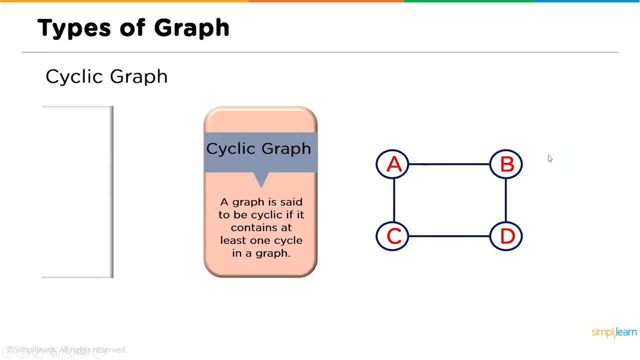 C to D, D to B and B to A again. So this type of a graph is called as a cyclic graph. Now, next we have the acyclic graph, So it is the typical opposite of the cyclic graph. So here: 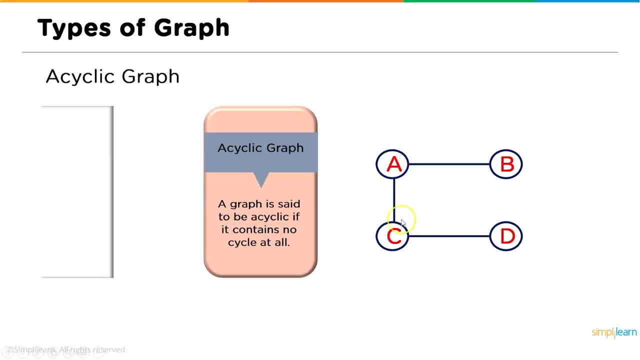 you cannot traverse to A again by traversing from A to C, C to D and there is no connection between D to B. So the complete cycle is not available here. This type of graphs are called as acyclic graphs. So, moving ahead, we have the graph representation. 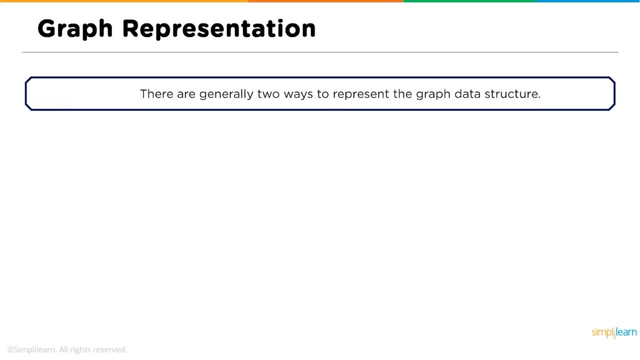 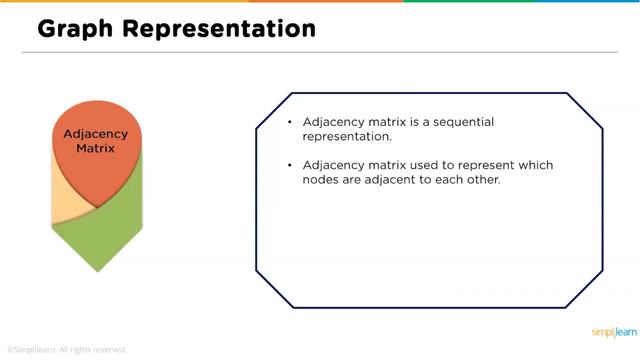 So generally, there are two different ways to represent the graph data structure. They are using adjacency matrix and adjacency list. So what is adjacency matrix? So adjacency matrix is a sequential representation. Adjacency matrix is used to represent which nodes are connected to which node, If there is an edge between two vertices. 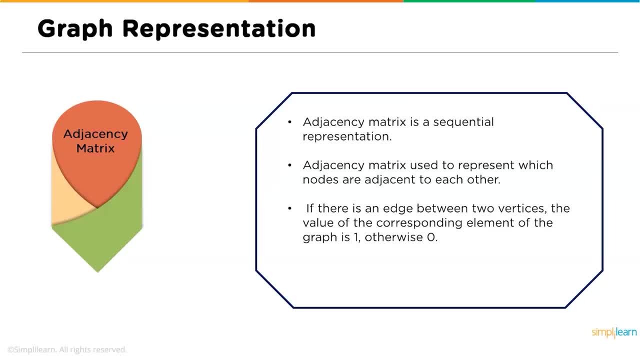 then the value of the corresponding element of the graph is one, Otherwise zero. If there is any weighted graph besides, then zeros and ones, we can store the weight of the edge as that particular number. Suppose that there is a connection between A and B and it is represented. 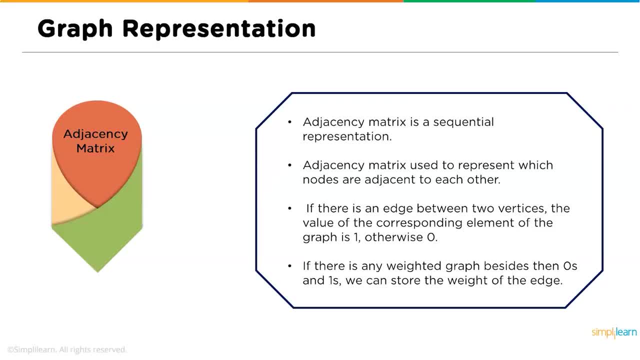 as a weight of five, then there is a connection. So we will use the connection as true, but we will not represent it as one. Instead, we will use the weight, that is five, to represent it as five, not as one. If there is no weight, then we will represent it as one, and if there is no connection, 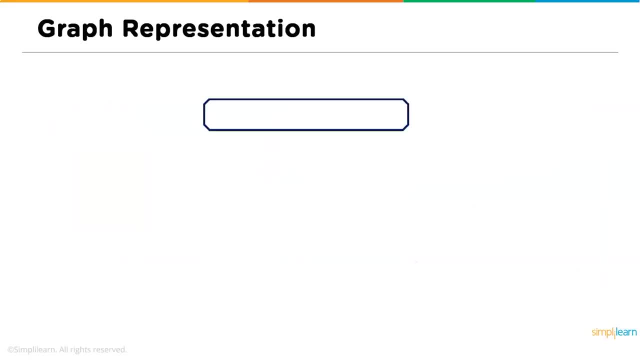 we will represent it as zero. Now undirected graph representation. So here you can see how we have represented a graph. So there is no connection between A to A, that is, there is no loop, so the value will be zero. 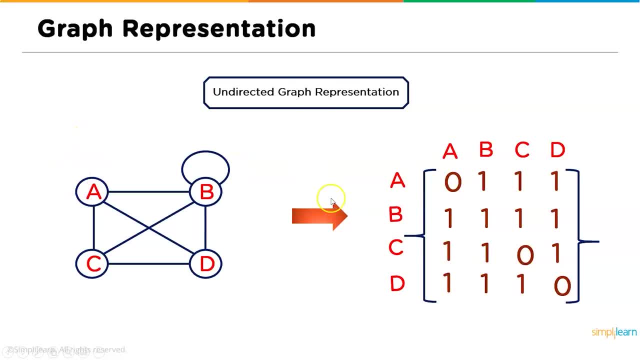 If there was a loop and if it was represented with a weight, then we could have written a weight here. Since we do not have weight, then the no connection is represented as zero and a connection is represented as one. We have a connection from A to B. 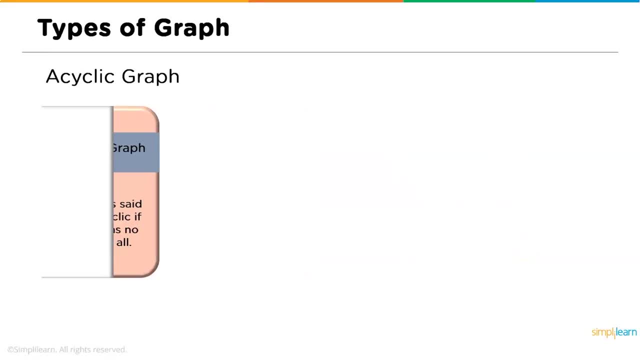 a cyclic graph. Now next we have the acyclic graph, So it is the typical opposite of the cyclic graph. So here you cannot traverse to A again by traversing from A to C, C to D, and there is no connection between D to B. So the complete cycle is not available here. This type of graphs. 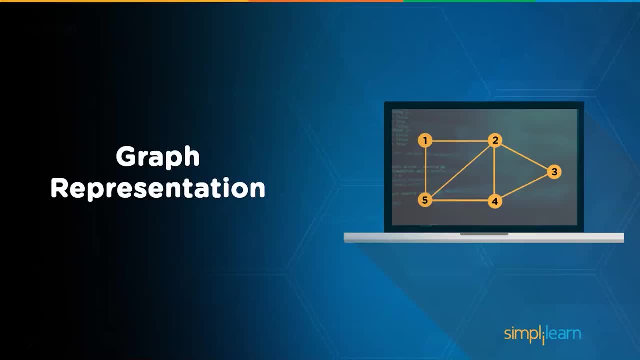 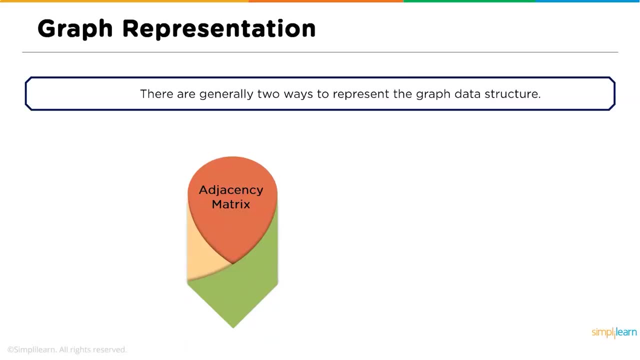 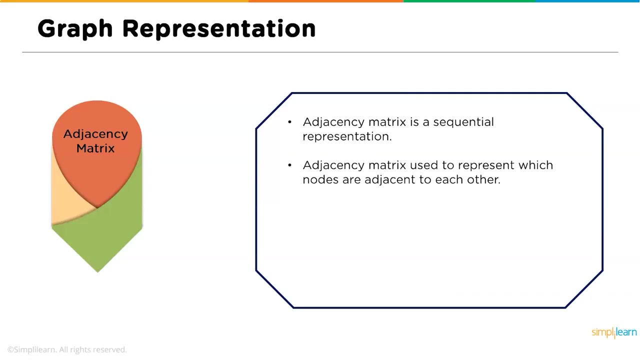 are called as acyclic graphs. So, moving ahead, we have the graph representation. So, generally, there are two different ways to represent the graph data structure. They are using adjacency matrix and adjacency list. So what is adjacency matrix? So adjacency matrix is a sequential representation. Adjacency matrix is used to represent which nodes. 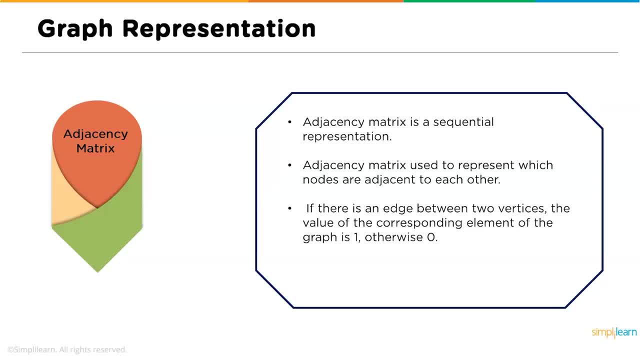 are connected to which node? If there is an edge between two vertices, then the value of the corresponding element of the graph is 1, otherwise 0.. If there is any weighted graph besides, then zeros and ones, we can say that the value of the corresponding element of the graph is 1.. 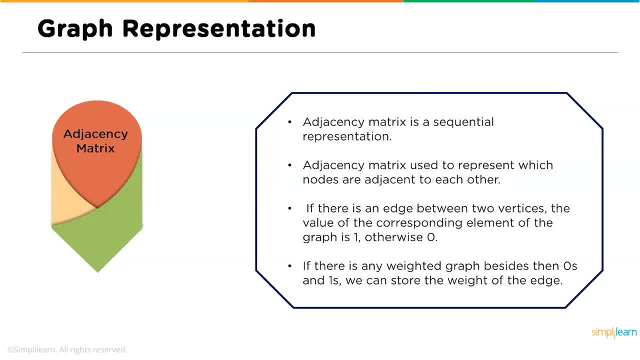 So we can store the weight of the edge as that particular number. Suppose that there is a connection between A and B and it is represented as a weight of 5. Then there is a connection. so we will use the connection as true, but we will not represent it as 1.. 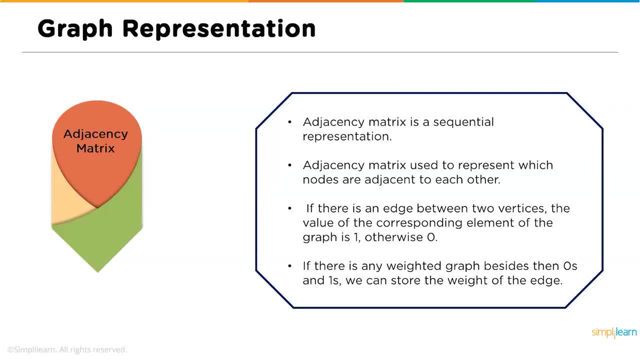 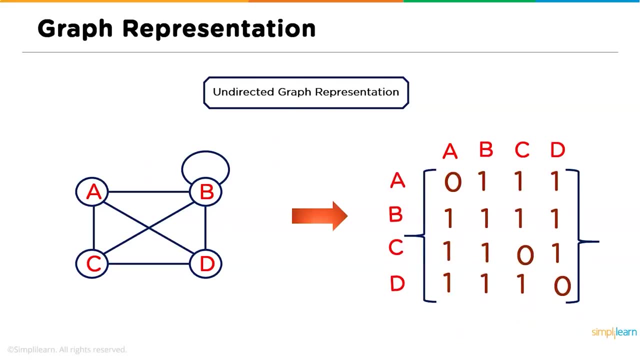 Instead, we will use the weight, that is, 5, to represent it as 5, not as 1.. If there is no weight, then we will represent it as 1, and if there is no connection, then we will represent it as 0.. Now undirected graph representation. So here you can see how we have represented a graph. 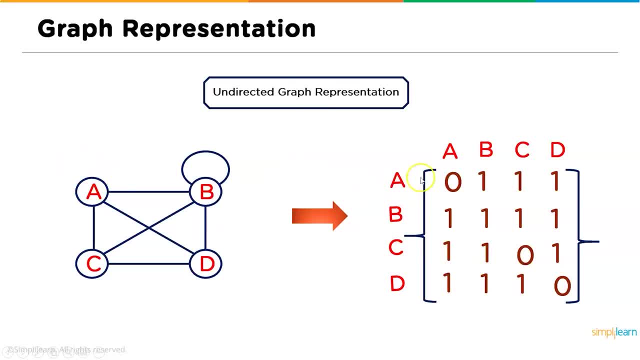 So there is no connection between A to A, that is, there is no loop. So the value will be 0.. If there was a loop and if it was represented with a weight, then we could have written a weight here. Since we do not have weight, then the no connection is represented as 0 and 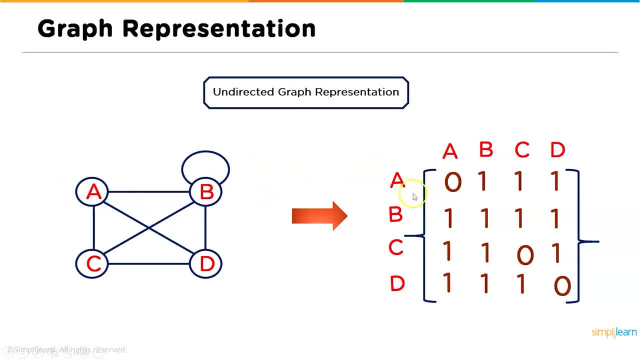 a connection is represented as 1.. We have a connection from A to B, so we have represented as 1, and similarly to A to C, so and so on. Now directed graph representation. So the simple difference between the directed and undirected graph representation is: we did not have a direction in the previous segment. 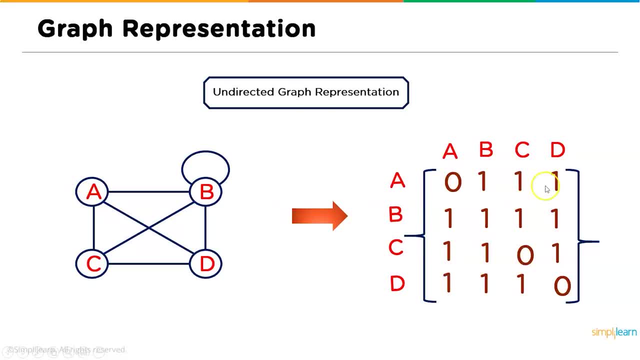 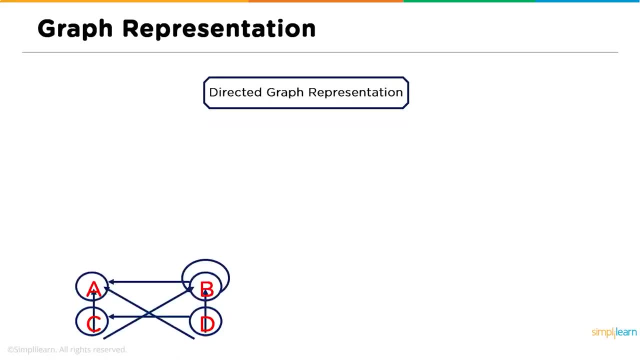 we have represented it as 1, and similarly to a to c, so and so on. Now directed graph representation. So the simple difference between the directed and undirected graph representation is we did not have a direction in the previous segment, but here we do have directions. So b is connected to a, but a is not connected to b, So we will write it as 0.. 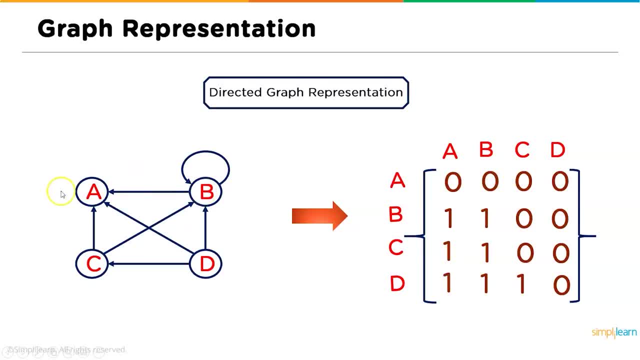 Because the control is traversing from b to a, but not from a to b. So we need to take care of the traversal of control. So we are represented as 0 and you can see, from d to b we have one connection and the traversal is in the direction of d to b, So we will have one there. So here we have d and b. 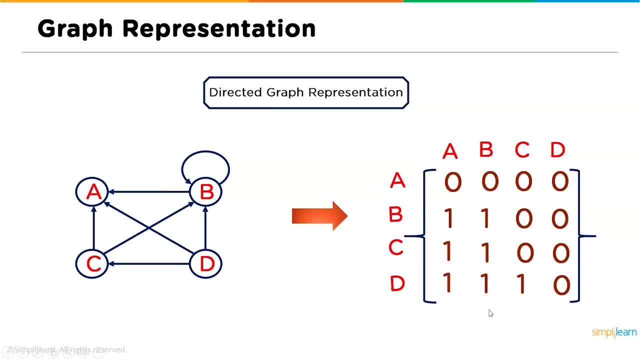 so we have one. So in that way we represent the directed graphs, Next undirected weight graphs. So this was what we discussed before: Instead of zeros and ones, we will represent the weight here. So we do not have a connection between a to a, So that is 0, as usual, but we do have a connection. 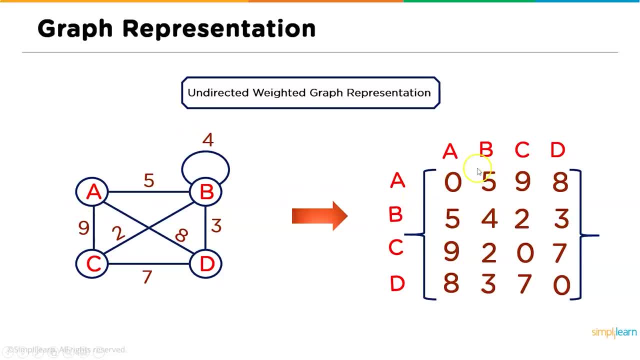 from a to b. So we have represented it with a number that happens to be the weight of the edge. And remember, we do not have the direction here. This is undirected weighted graph. Now, if it were the directed weighted graph, then we could have seen the direction and represented 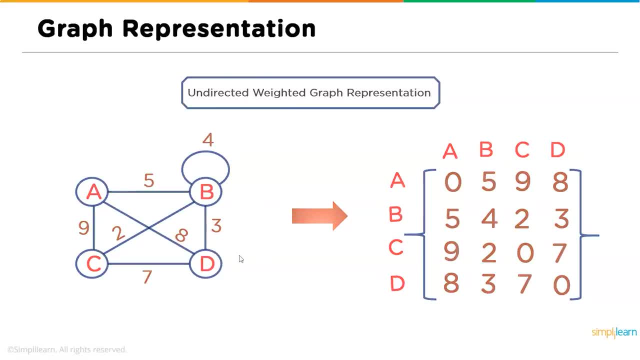 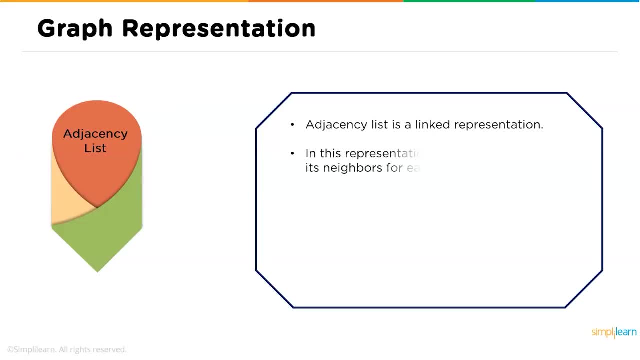 number with the weight. Now, after this, let us look into the adjacency list. So what is adjacency list? Adjacency list is a linked representation. In this representation, we maintain the list of its neighbors for each vertex in the graph. Every vertex of the graph contains the list of adjacency vertices, Array of vertices which 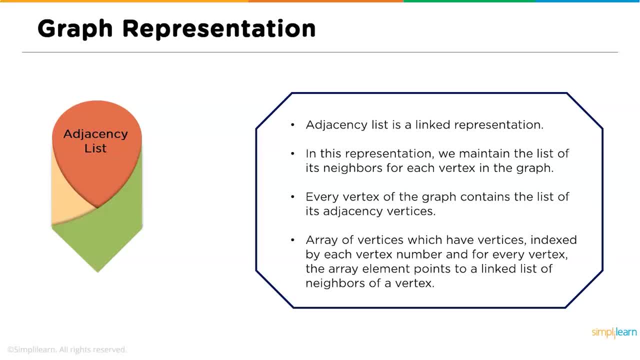 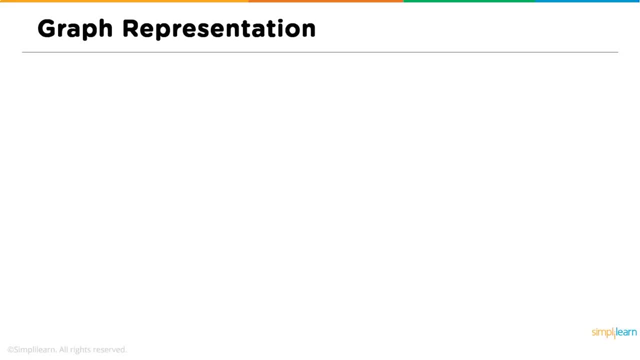 have vertices indexed by each vertex number. for every vertex, The array element points to the linked list of the neighbors of the vertex. So this might be a little complicated to understand. So let us understand this using an example. So directed graph representation implemented using 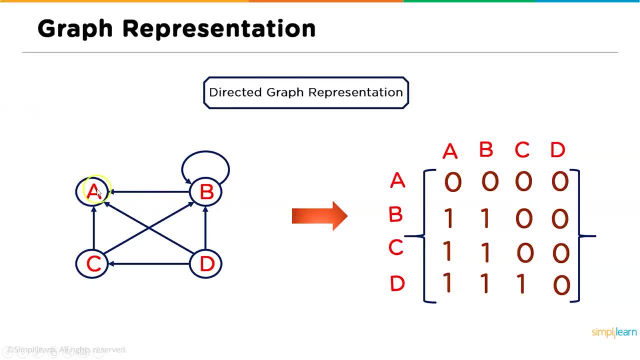 but here we do have directions. So B is connected to A, but A is not connected to B. So we will write it as 0, because the control is traversing from B to A but not from A to B. So we We need to take care of the traversal of control. 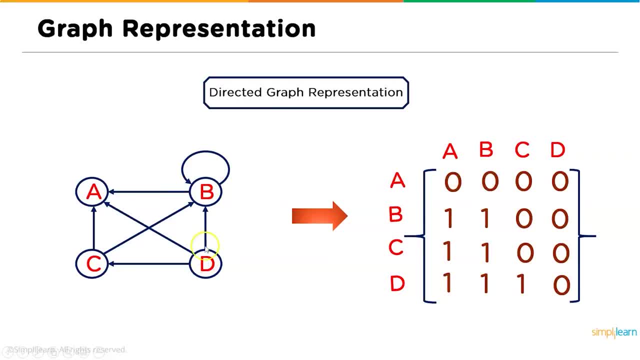 So we are representing as zero. and you can see, from D to B, we have one connection and the traversal is in the direction of D to B, So we will have one there. So here we have D and B, So we have one. 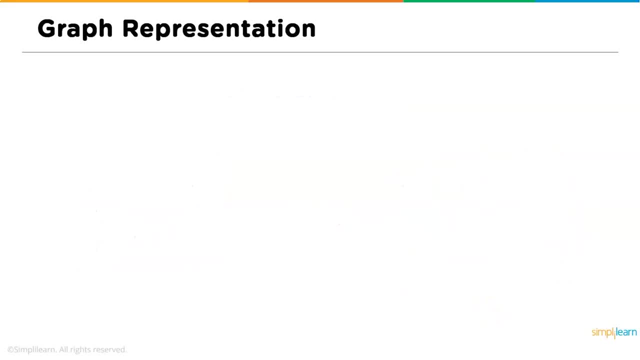 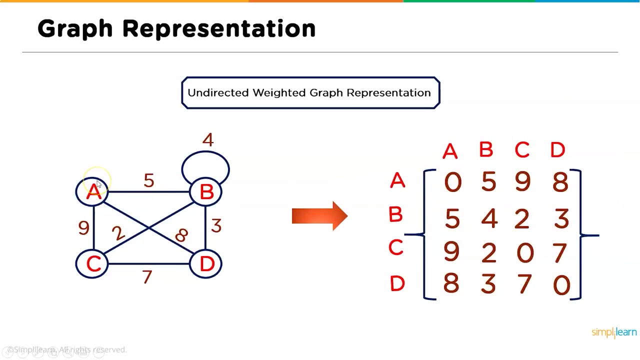 So in that way we represent the directed graphs, Next undirected weight graphs. So this was what we discussed before: Instead of zeros and ones, we will represent the weight here. So we do not have a connection between A to A, So that is zero, as usual, but we do have. 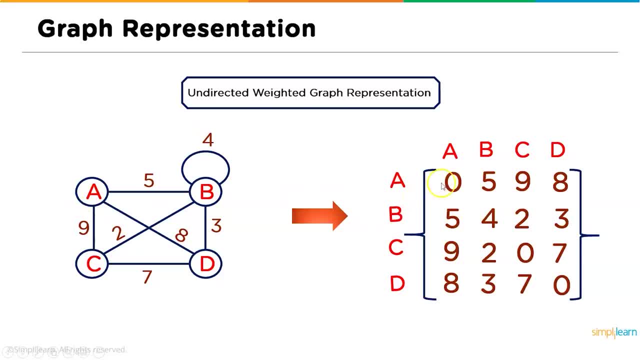 a connection from A to B. So we have represented it with a number that happens to be the weight of the edge. And remember, we do not have the direction here. This is undirected weighted graph. Now, if it were the directed weighted graph, then we could have seen the direction and 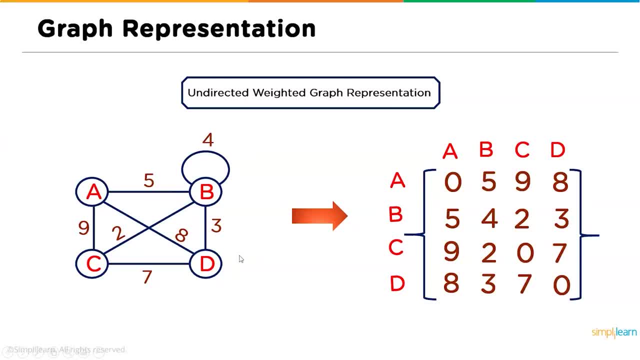 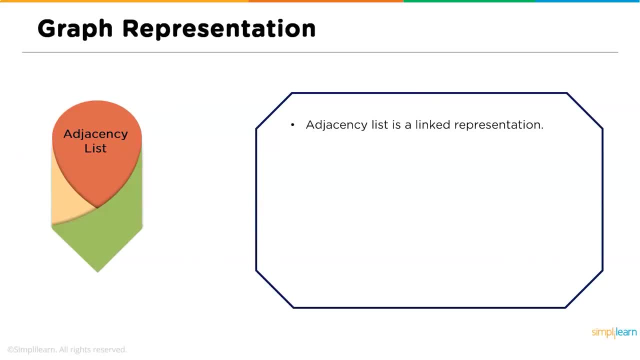 represented the number with the weight. Now, after this, Let us look into the adjacency list. So what is adjacency list? Adjacency list is a linked representation. In this representation, we maintain the list of its neighbors for each vertex in the graph. 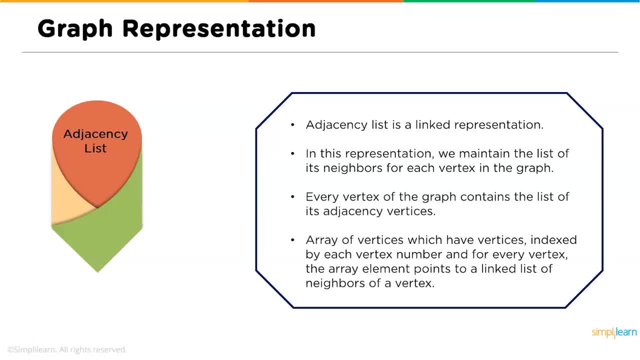 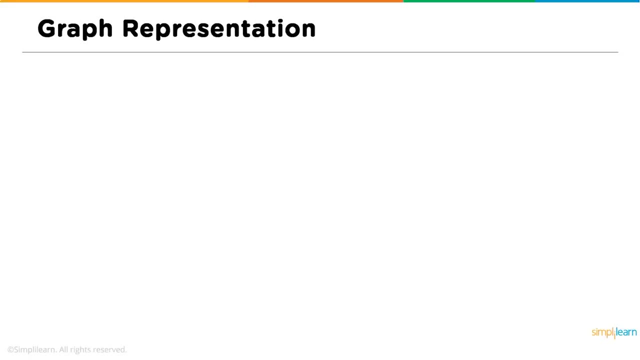 Every vertex of the graph contains the list of adjacency vertices: Array of vertices which have vertices indexed by each vertex number. for every vertex, The array element points to the linked list of the neighbors of the vertex. So this might be a little complicated. So let us understand this using an example. 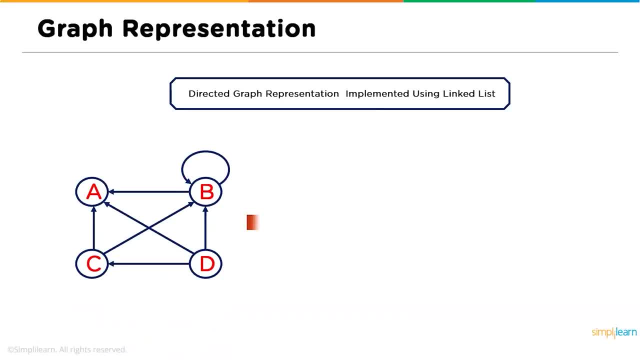 So directed graph representation implemented using linked list. So this is the directed graph we are using. So you can see that A is not connected to anything. So we have ended the address of next location as X, But B is connected to A and C is connected to A. Similarly, D is also connected to A. 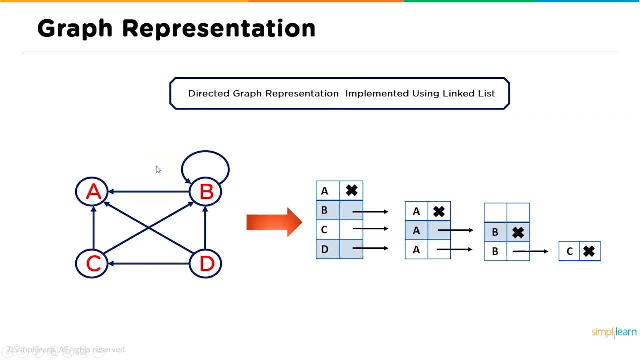 So that is how we represent the directed graphs, using linked list. Next, we have directed graph representation using array. So A is not connected to anything, So we have represented as 0.. And B is connected to B and as well as A, So we have 1 there. 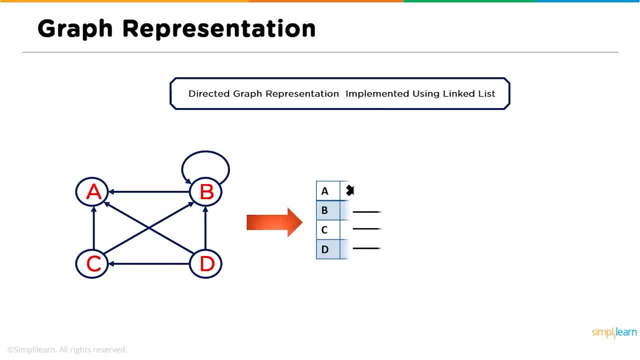 linked list. So this is the directed graph we are using. So you can see that a is not connected to anything. So we have ended the address of next location as x, but b is connected to a and c is connected to a. Similarly, d is also connected to a. So that is how we represent the. 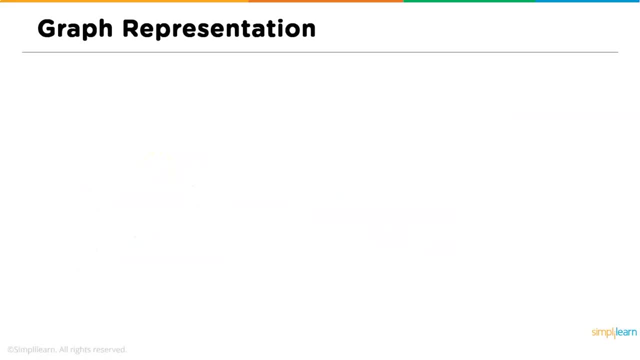 the directed drafts using linked list. Next, we have directed graph representation using array. So a is not connected to anything. So we have represented as zero and b is connected to b and as well as a, So we have one there and c is connected to b. 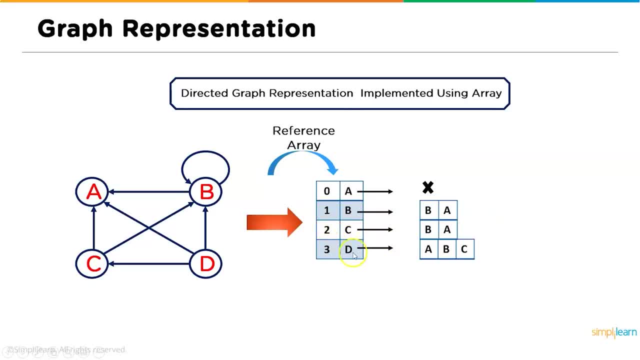 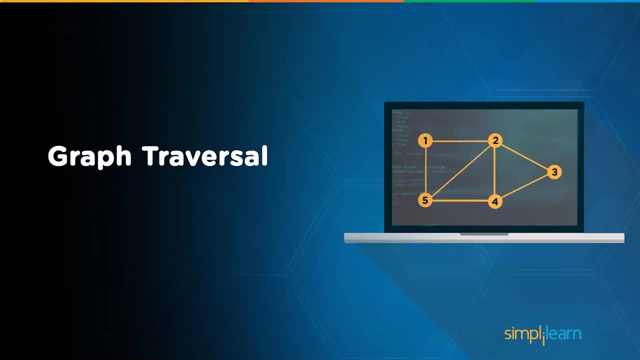 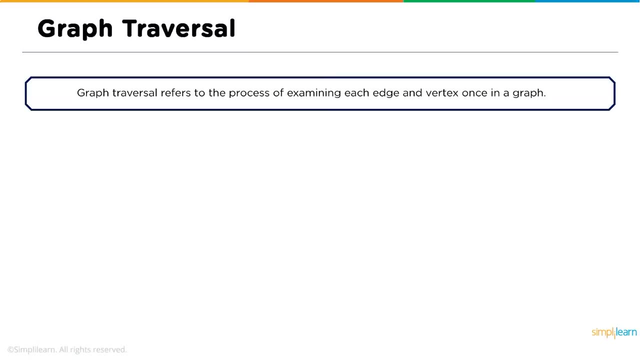 So c is also connected to a, So we have two there. d is connected to a, c and b, So we have three there. Now we have the graph traversal. So graph traversal refers to the process of examining each edge and vertex in a graph. 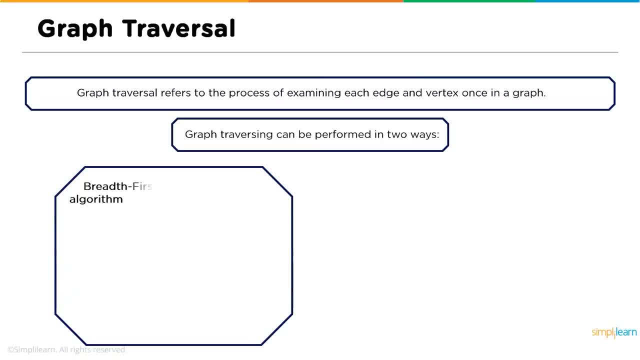 Graph traversing can be performed in two ways. The first one is breadth-first search or BFS algorithm. BFS starts traversing the graph from root node and explores all the neighboring nodes, Then it selects the nearest node and explores all the neighboring nodes, Then it selects the nearest. 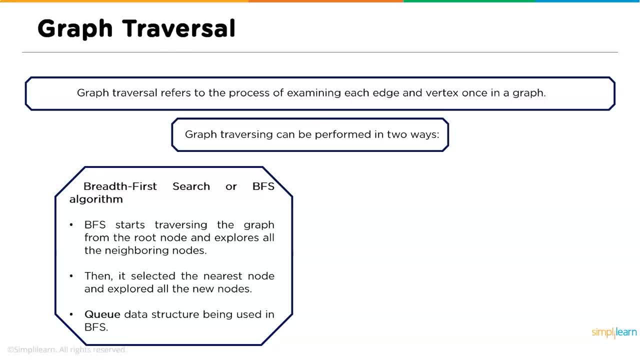 all the new nodes. Queue data structure can be used in BFS algorithm. So the following image depicts the BFS algorithm working. It chooses the nearest node first, then it traverses to all the other nodes, So, followed by BFS algorithm, we have the DFS algorithm. that is the depth first. 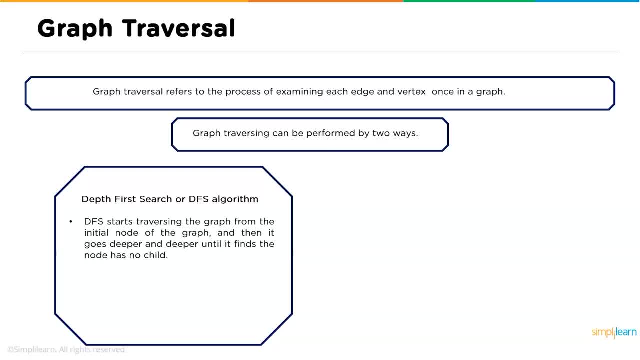 search algorithm DFS starts traversing a graph from the initial node of the graph and then it goes deeper and deeper until it finds the node has no child. Then backtrack from the dead end towards the recently explored nodes. Stack is used for BFS algorithms, So this particular GIF image. 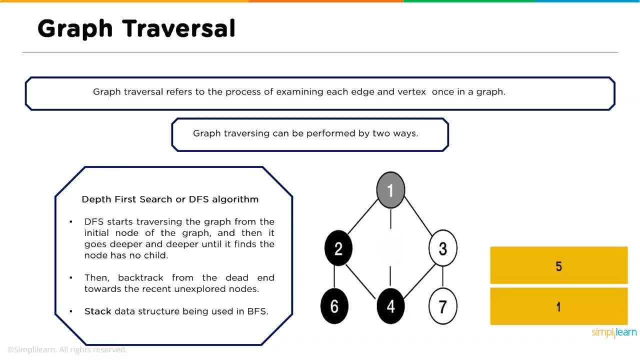 can be considered as the graph traversal which is performed using DFS algorithms. So if you don't know much about DFS and BFS algorithms, don't worry about that. Those particular tutorial videos are added in the description box below. You can go through it and understand BFS and DFS algorithms. 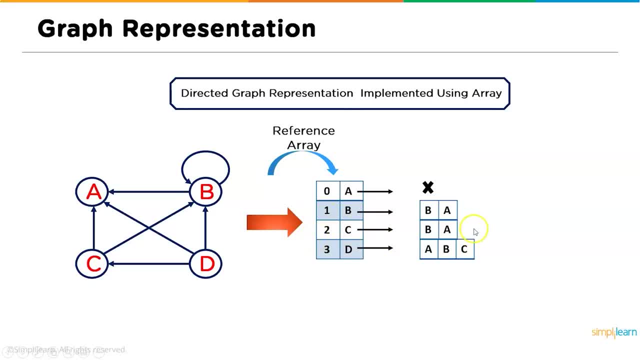 And C is connected to B, So C is also connected to A, So we have 2 there. D is connected to A, C and B, So we have 3 there. Now let us look into the array. Now we have the graph traversal. 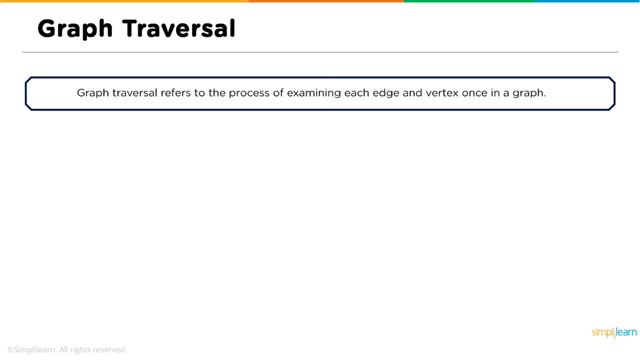 So graph traversal refers to the process of examining each edge and vertex in a graph. Graph traversing can be performed in two ways. The first one is breadth-first search, or BFS algorithm. BFS starts traversing the graph from root node and explores all the neighboring nodes. 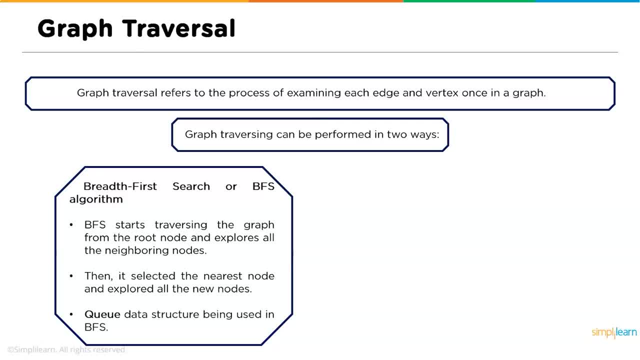 Then it selects the nearest node and explores all the new nodes. Queue data structure can be used. So the following image depicts the BFS algorithm working. It chooses the nearest node first, then it traverses to all the other nodes, So, followed by BFS algorithm, we have the DFS algorithm. that is the depth-first search. 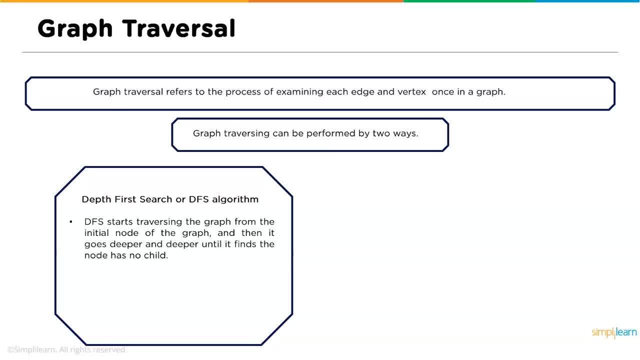 algorithm DFS starts traversing a graph from the initial node of the graph and then it goes deeper and deeper until it finds the node has no child. Then backtrack from the dead end, Then backtrack towards the recently explored nodes. Stack is used for BFS algorithms. 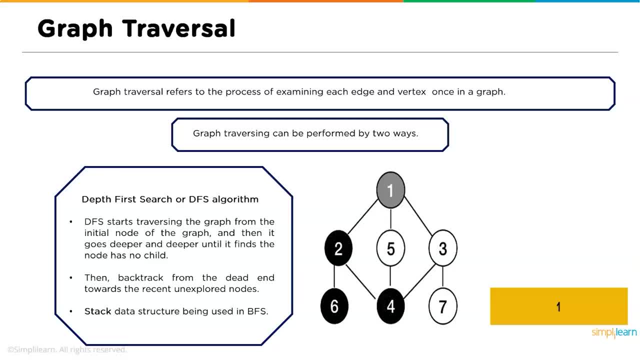 So this particular GIF image can be considered as the graph traversal which is performed using DFS algorithms. So if you don't know much about DFS and BFS algorithms, don't worry about that. Those particular tutorial videos are added in the description box below. You can go through it and understand BFS and DFS algorithms in a much better way. 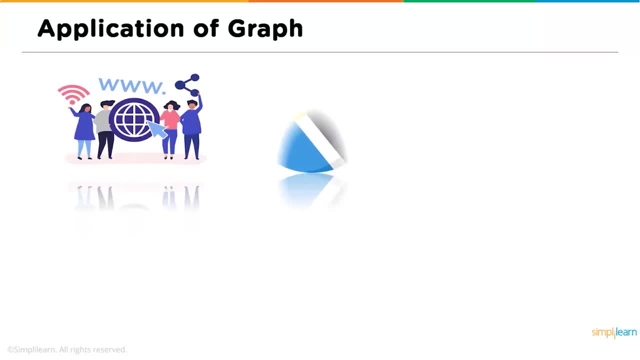 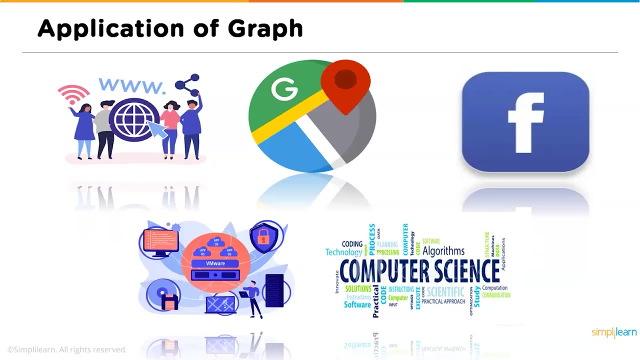 Now we will go through some of the applications of graphs. So Some of the major applications of graphs are used in the websites Google Maps and social media websites like Facebook, and some security systems and also software programming. So with that we have come to an end of this tutorial. 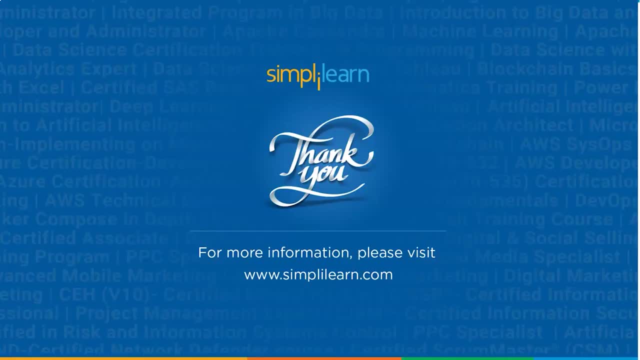 If you have any queries regarding the topics discussed in this particular tutorial, then please feel free to let us know in the comment section below, and our experts will be happy to solve all your queries. Until next time, thank you, stay safe and keep learning. 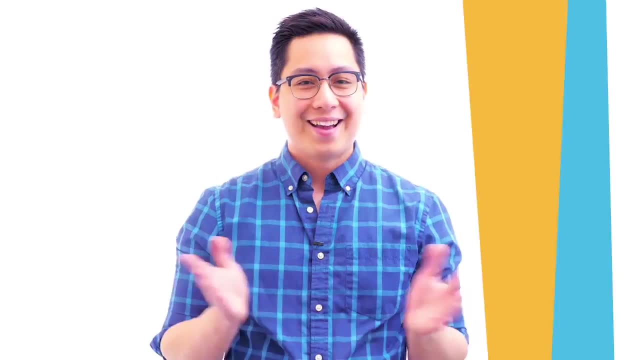 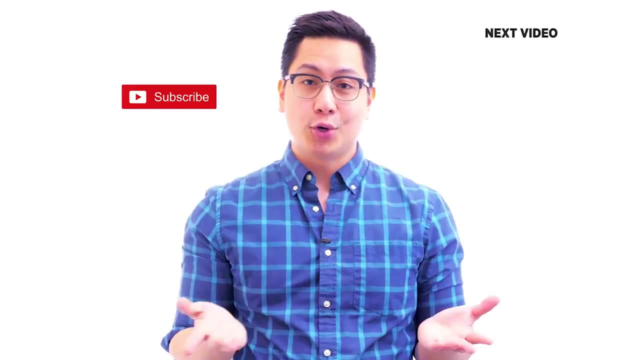 Hi there. if you liked this video, subscribe to the Simply Learn YouTube channel and click here to watch similar videos. To nerd up and get certified: click here.